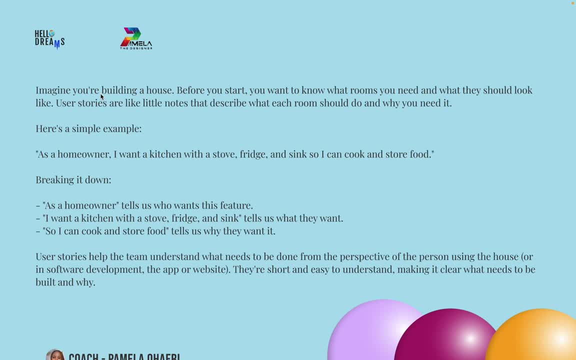 homeowner, I want a kitchen with a stove, a fridge, a sink, so that I can cook and store food. So let's break it down: As a homeowner, this tells us, or this tells you, who wants the future. A homeowner, someone who is going to be the home owner, right? So I want a kitchen with a stove. 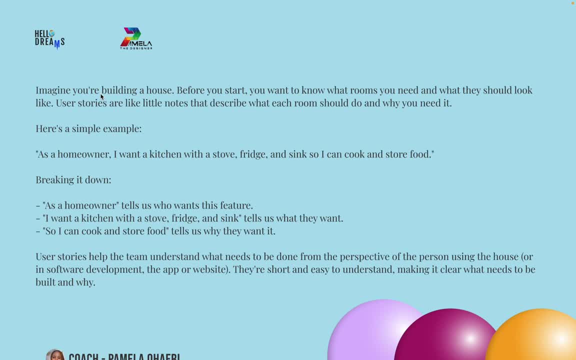 fridge and sink. This particular section tells us what they want, what the homeowner wants, So I can cook and store food. This part tells us why they want it. So user stories help the team in an agile thing or help anyone building a product to understand what needs to be done from the 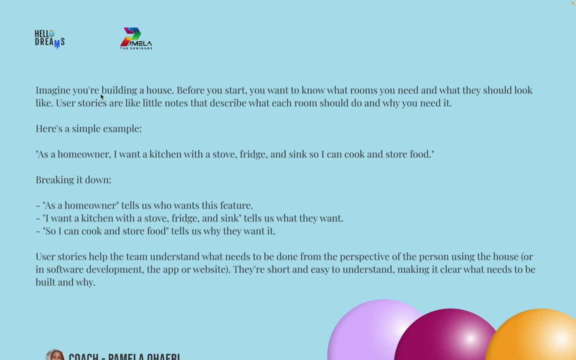 perspective of the person using that product, using the house or in a software development app or website. They are like short and easy to understand. It's also written in a way that it is clear, so that what needs to be done or what needs to be built is understood, and why we need to build. it So I can cook and store food. This part tells us why they want it. So user stories help the team in an agile thing or what needs to be done, or what needs to be done from the perspective of the person using the house, fridge and sink. This particular section tells us what they want, what the homeowner wants. 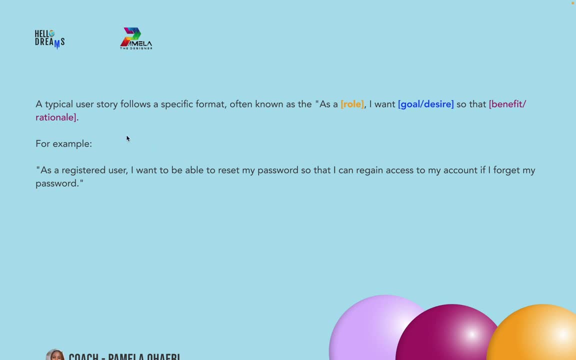 is also understood, All right. so a typical user story follows a specific format, often known as the as a, which is a role, the person I want, your goal, your desire, so that the benefit, the rationale. So this is another example. As a registered user, I want to be able to reset my 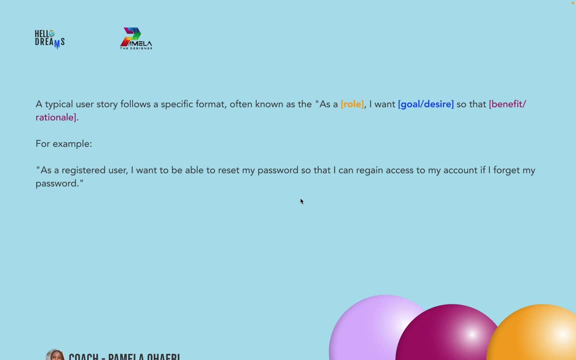 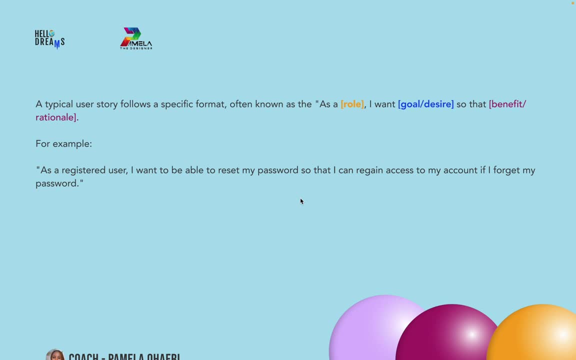 the registered user right. who wants? what do they need? what's their goal? their desire is to be able to reset their password. why? what's the benefit? so that they can regain access to the account if they forget their password. all right, so user stories are written in this format. 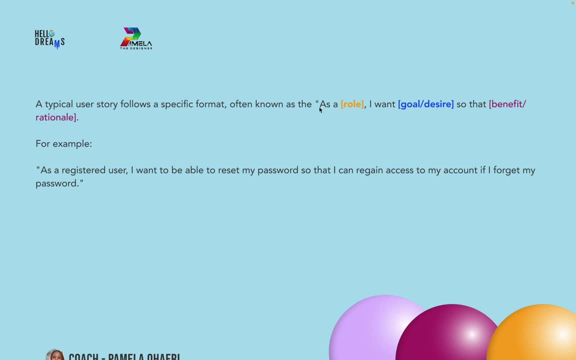 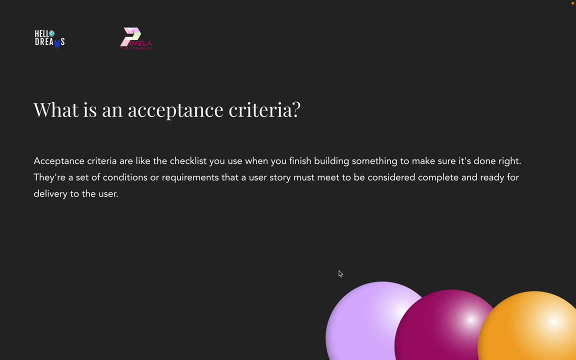 the role, the person, what they want and the benefit or rationale behind it. so let's look at what is an acceptance criteria? what acceptance criteria is? acceptance criteria are like the checklist you use when you finish building something to make sure it is done right, their set of conditions or requirements that a user story must meet to be considered. 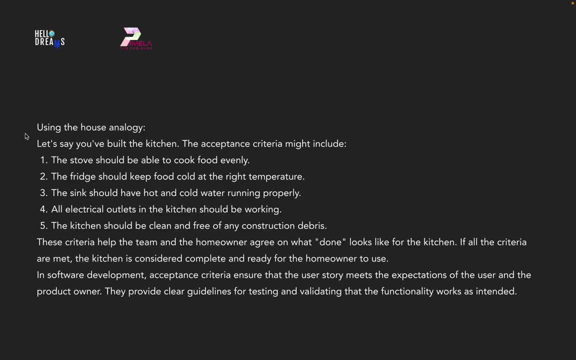 complete and ready to be delivered to the user. so this is an example. let's use the analogy of the house. let's say you have built the kitchen. the acceptance criteria might include: the stove should be able to cook food evenly, so on. unless that stove is able to cook, you have not met the 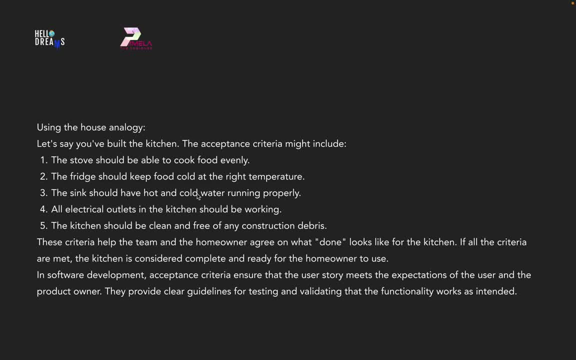 criteria of the user. story two: the fridge should keep food cold at the right temperature. three, the sink should have hot and cold water running properly. all electrical outlets in the kitchen should be working. the kitchen should be clean and free of all construction debris. this criteria helped the team, so in essence, this: 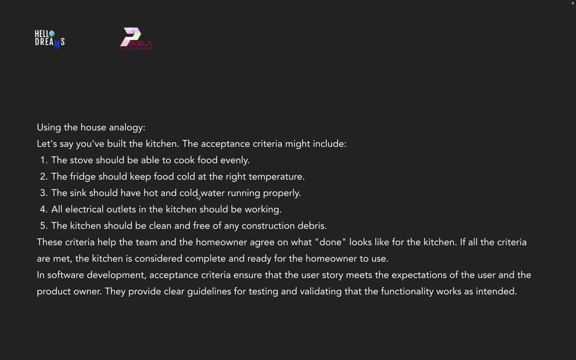 criteria helped the team and the homeowner agree on what done looks like for the kitchen. if all the criteria are met, the kitchen is considered complete and ready for the homeowner to use. so in In software development, acceptance criteria ensure that the user meets the expectation of the user and the product's owner. 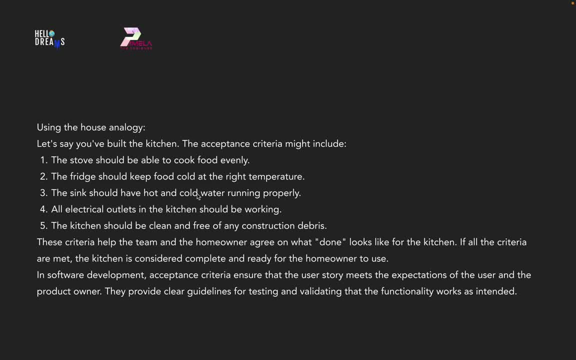 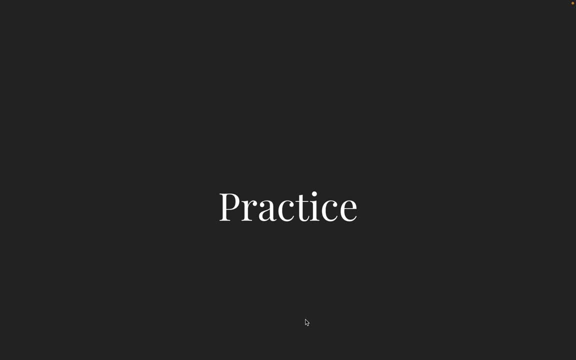 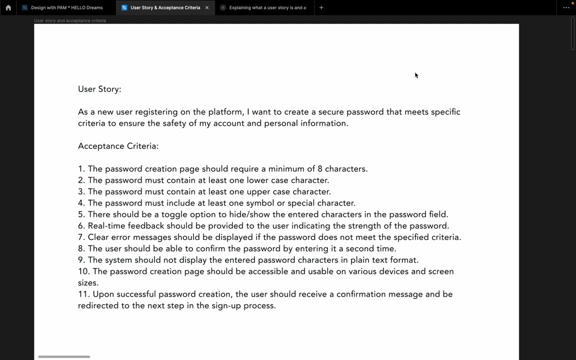 They provide clear guidance for testing and validating that functionality works as intended. Alright, so let's move on to practice this. We're going to read a user story and then design it proper in Figma. Let's get into it. This is what a user story is. 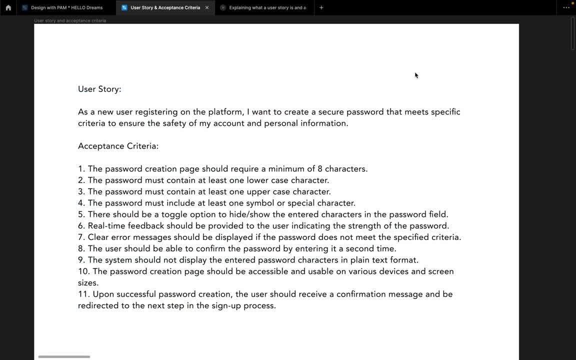 This is what we're going to be treating, what we're going to be designing. So it says: as a new user registering on the platform, I want to create a secure password that meets specific criteria to ensure the safety of my account and personal information. 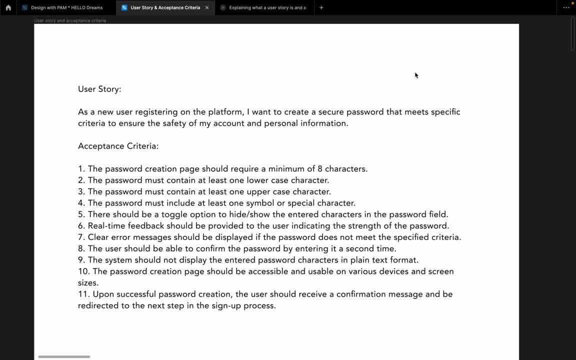 That's the user story. Now, this is the acceptance criteria: 1. The password creation page should require a minimum of 8 characters. 2. The password must contain at least one lowercase, 3. One uppercase character, 4. One symbol or special character. 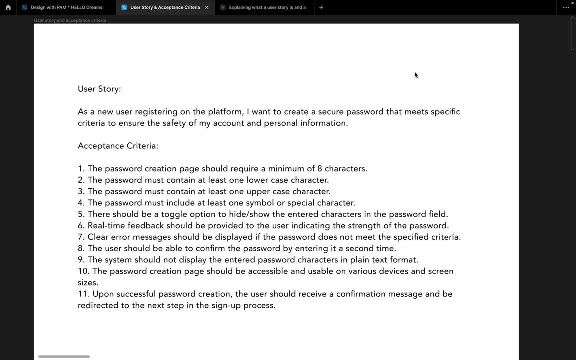 5. There should be a toggle option to hide or show the entered characters. 6. Read time feedback should be provided to the user, indicating the strength of the password. 7. Clear error messages should be displayed if the password does not meet the specific criteria. 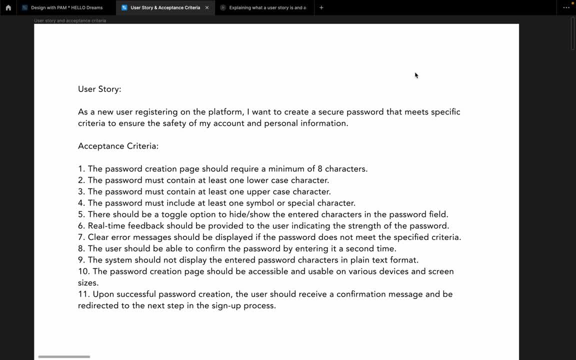 8. The user should be able to confirm the password by entering it a second time. 9. The system should not display the entered password characters in plain text. 10. The password creation page should be accessible and usable on various devices and screen sizes. 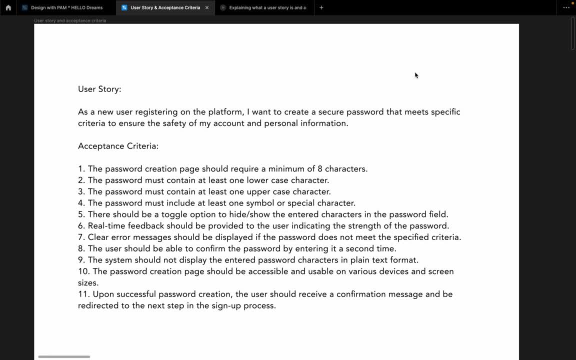 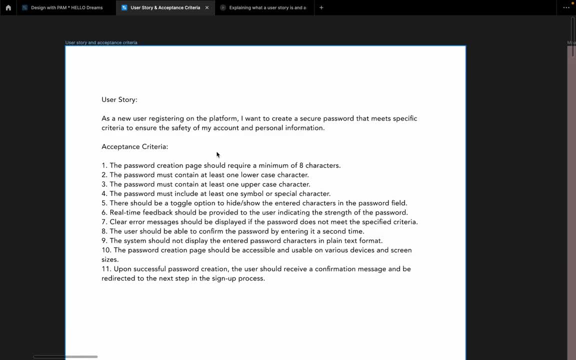 11.. Upon successful password creation, the user should receive a confirmation message and be redirected to the next step in the sign-off process. Alright, so we're going to go right into it. This is what a typical user story looks like, right? 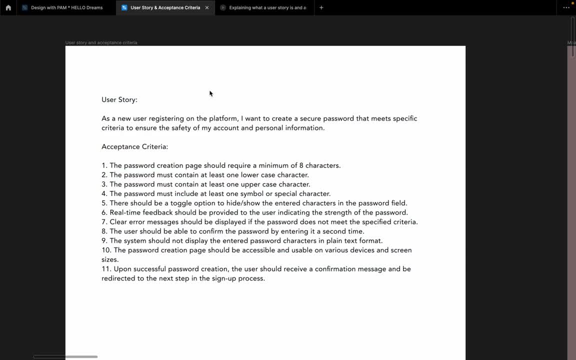 As a designer, you get to design the interface and the development team brings it to life right. So there's a certain aspect of the user story that speaks specifically to developers and some that you must implement on the interface. So there's a certain aspect of the user story that speaks specifically to developers and some that you must implement on the interface. 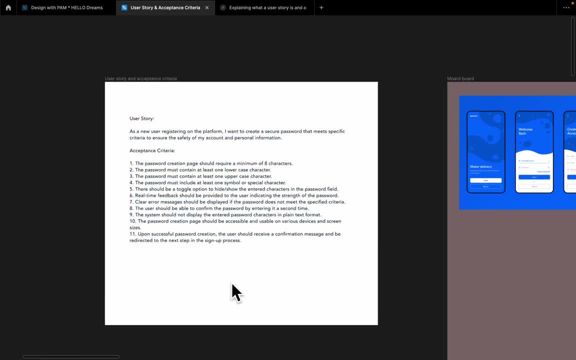 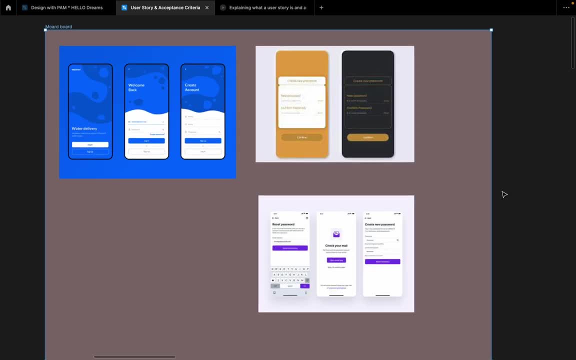 Alright, so what? we're going to implement almost everything here, But before we start, I just want you to know that, as a designer, it doesn't necessarily mean that when you open your canvas to design, that you know everything and you can just start designing. 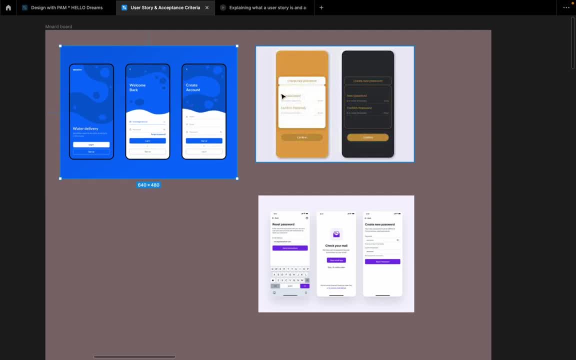 We work with Moodboard, So I just typed maybe login screen, sign up screen on Google. I use Google, I use Pinterest, I use Dribbble, I use Behance, I use Mobbing to find inspiration on my designs. 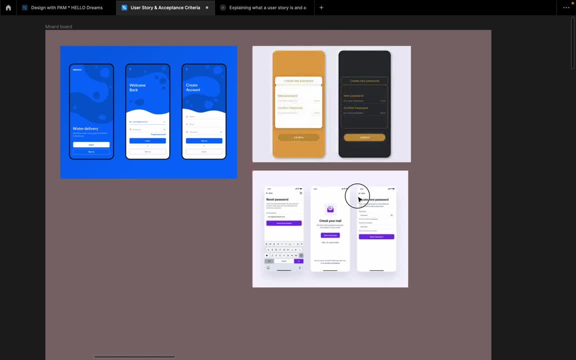 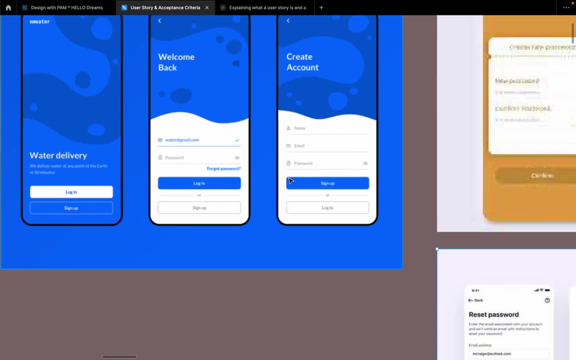 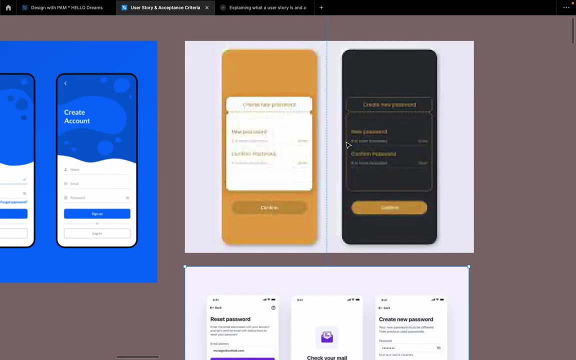 designs, right. so these are the key things that i found from um this site, and i think i like the screen, i like the blue thing going on here, though this is not a typical creation and password creation page, right, but i can still pick one or two inspiration from here. this is also um. this is. 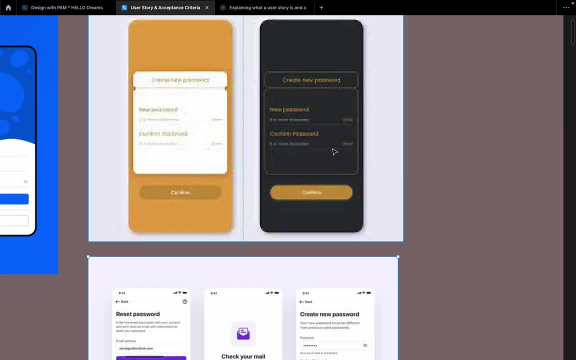 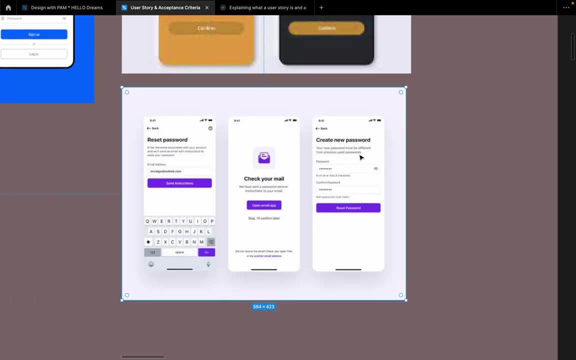 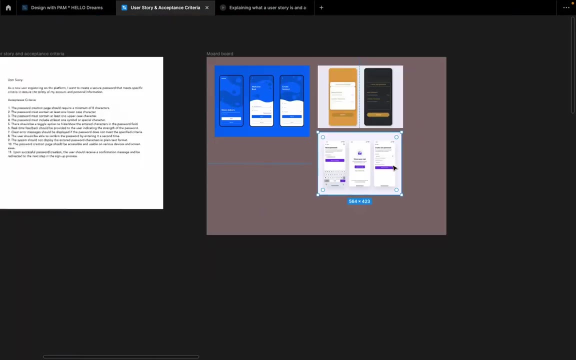 also something i can work with. i think when i saw it online it was clearer than this, but again, i think i already got the inspiration i needed from it. then this one also can also help. okay, so, as you can see, there's a a portion of this story that says that let's look at this. the system should. 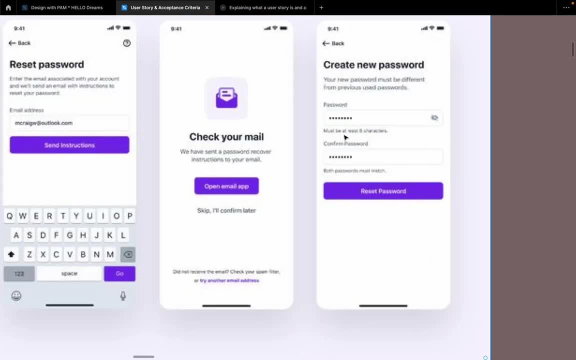 not display the entered password characters in plain text. so, as you can see here, this password that you've entered is not in plain text to show what you have. so you have this toggle here where you can see it, or you should not see it. so let's get right into it now that we have our mood board. 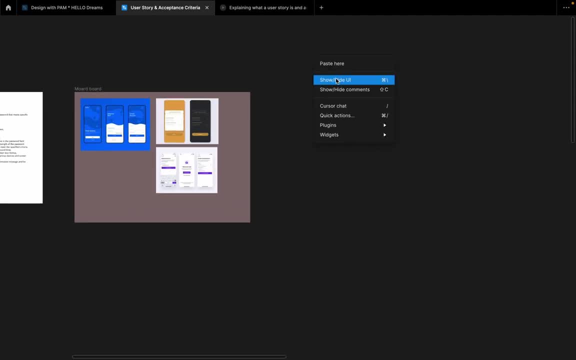 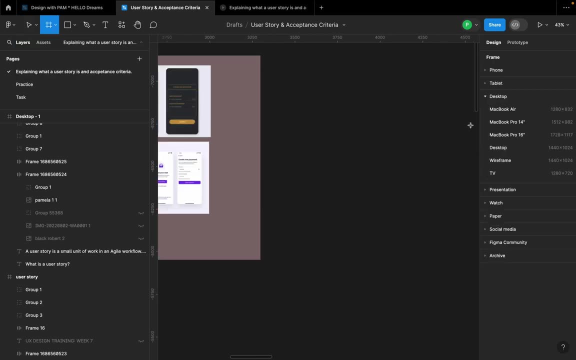 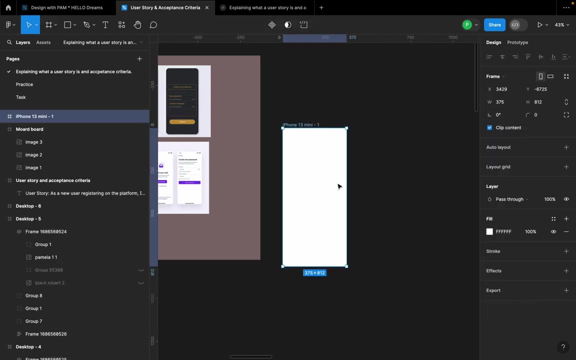 let's start with the mood board designing. so i'm going to go back and bring out the show- our ui here i am going to come here- or just short form: just click f on your keyboard. you're going to see these options here on your right hand side, this properties panel. i'm going to select the iphone 13 mini, what i'm going to do. 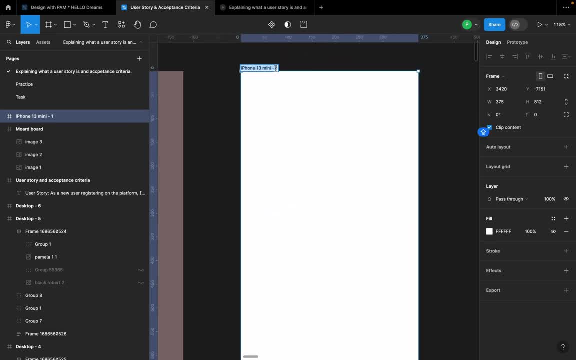 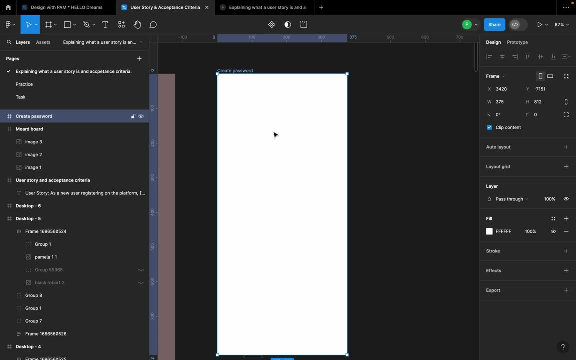 is, i am going to tie to my frame to be create password. so the next thing: again, we need to work with grid lines. so i'm going to go back and i'm going to go back, and i'm going to go back and i'm going to show you again. i'm going to go on your smartphone. what i'm going to do is set up the. 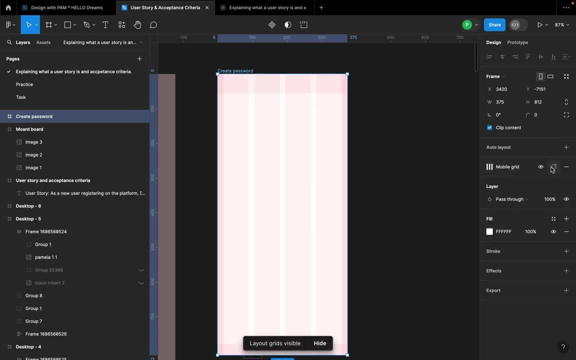 grid lines so that we're sure of what we're doing. i already have my mobile grid lines here, so i'm going to detach this down so you can see the settings. you can just copy out the settings here. from here you can apply the same settings. if you have one that is working for you, that is good. 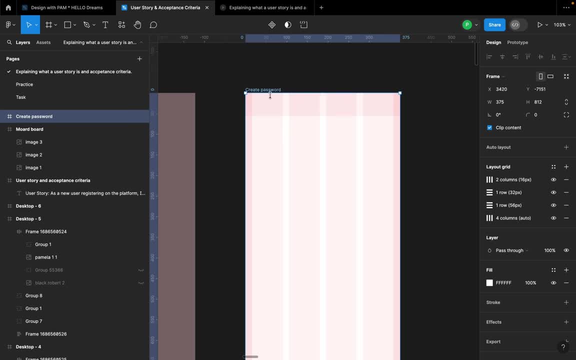 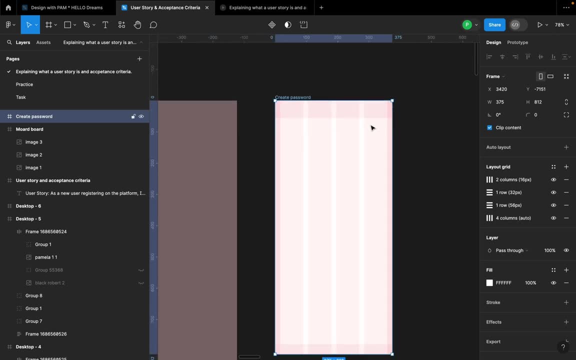 alright. so what we're going to do now, you remember, on um every mobile screen, there's usually a space for where you see your timer, where you see your battery percentage, your wi-fi. so what we're going going to do is we're going to create a space for that. so i'm going to click on my keyboard, or rather, 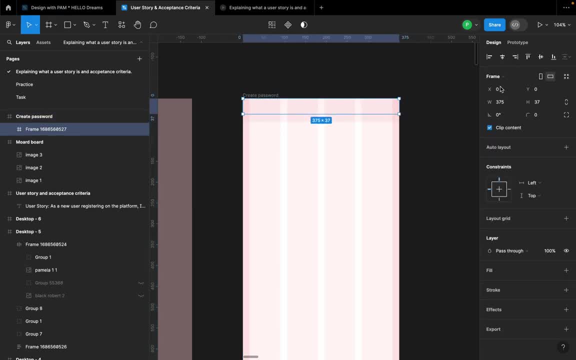 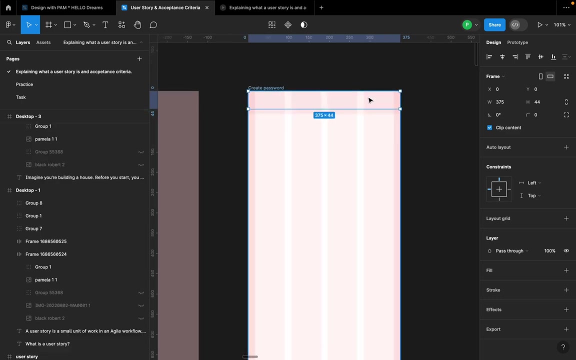 go to this frame and i'm going to draw a tiny frame here. i'm going to give the height a 44, 44 is okay, right? so this is where i'm going to. i'm making provision for it here. i already have those items copied on my clipboard. the items are copied on my clipboard, so i'm going to hit. 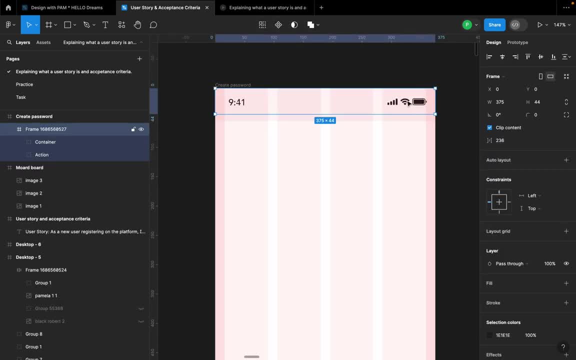 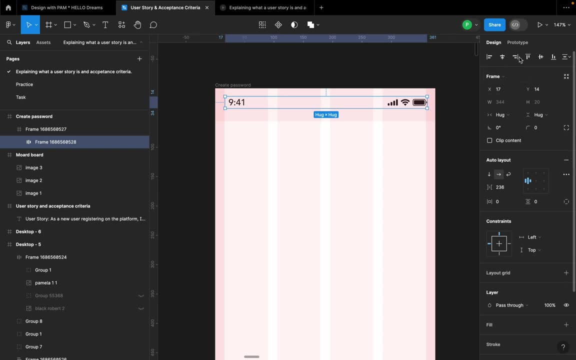 ctrl v or command v to paste it here. i'm going to select the two. create an auto layout, because i want it to align properly. then i'm going to come to this alignment section. here i'll make sure that it is aligned vertically in the frame where i placed it in, and i'm also going to make 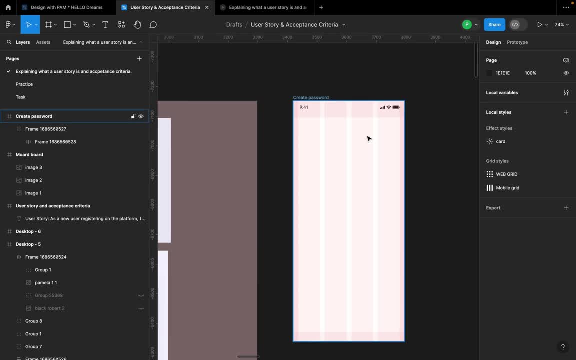 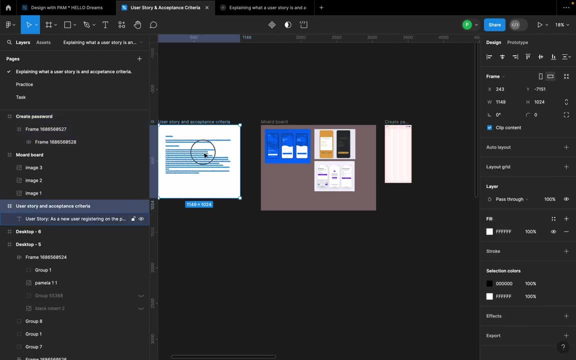 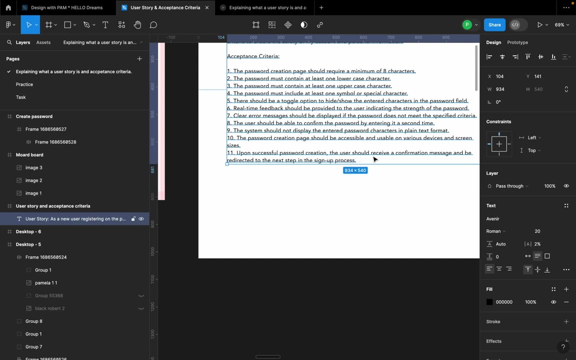 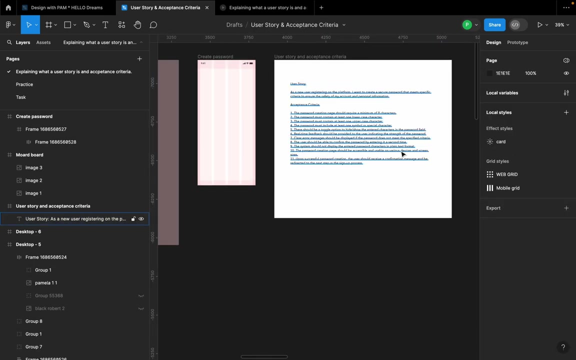 sure that it is aligned horizontally. this is fine. this kind of page we have like a, a progress bar. you remember that? this acceptance criteria here, let's bring it here, you, at the end of this acceptance criteria, it says: upon successful password creation, the user should receive a notification message and be redirected to the next step in the signup process. normally. 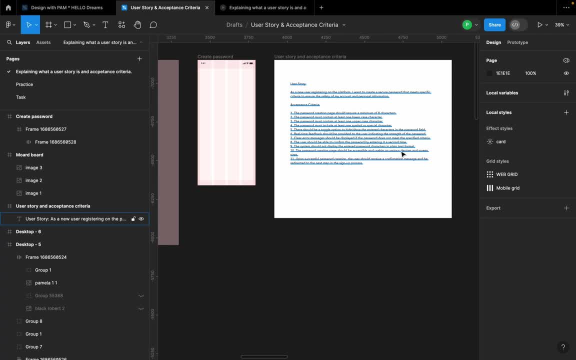 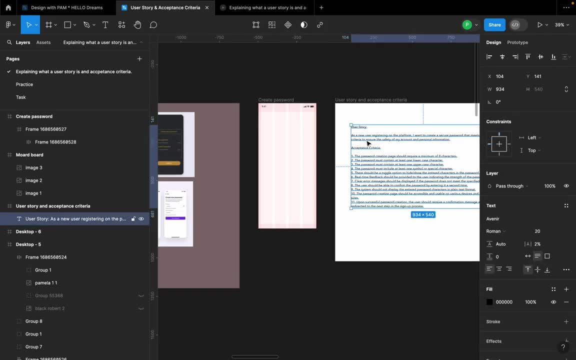 for most of the signup processes that i've seen, creating password is mostly the last stage after you've provided your information. i'm going to assume that this is the last stage for this user story and acceptance criteria. i am going to create like a progress bar thing going on. 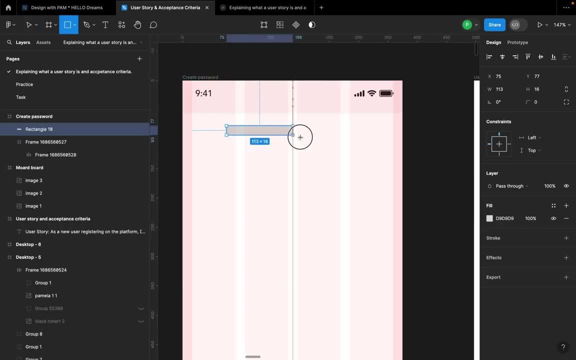 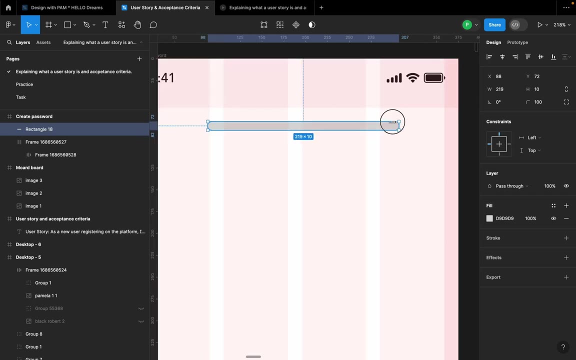 here. so i'm going to hit r on my keyboard and draw a tiny rectangle. i'm going to make it just very small. the height is: let's give the height a 10, which is fine. i'm going to round the corners to up to 100 because i want it very rounded. let's reduce this just a bit. 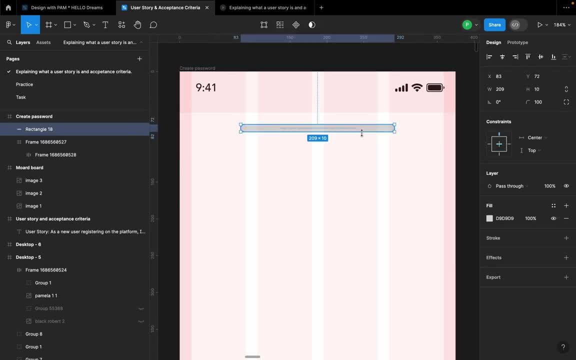 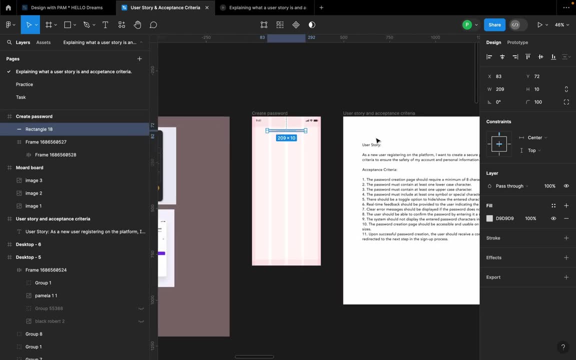 make sure this is centered here. i want to be sure this is not too big, okay so. So another thing I'm doing here: I'm going to be using a color I like- blue, So I'm going to make sure that the dominant color here, my primary color, is blue. 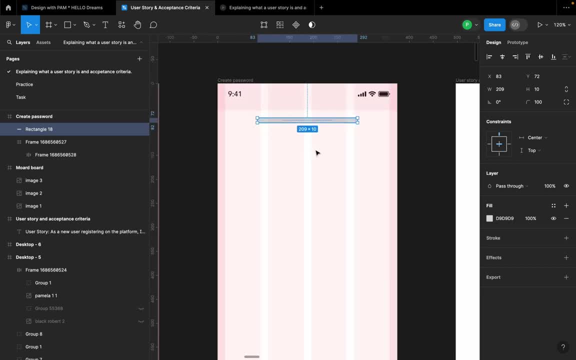 Remember I told you that I like the blue concept. here Again, choosing color for your design is not just up to you. You need to consult with the brand. What is your primary color? What are the colors of their choice? That is what determines the color you're going to be using. 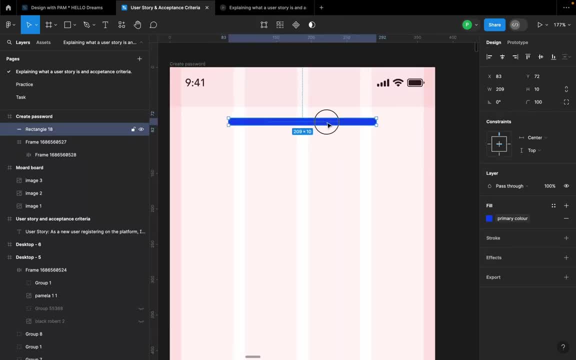 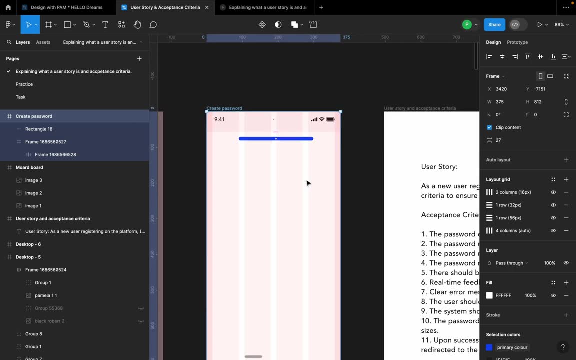 But I have my primary color here, So I'm going to select it. This is fine For my back button. what I'm going to do, I already have it copied on my clipboard, So I'm just going to paste it. If you don't have a back button, just click on right click on your mouse. 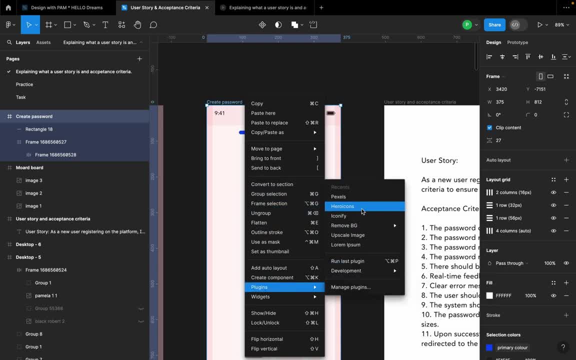 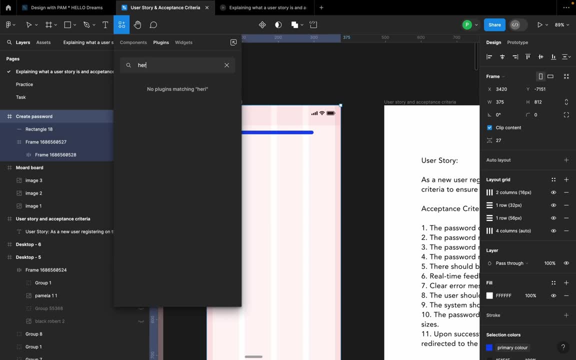 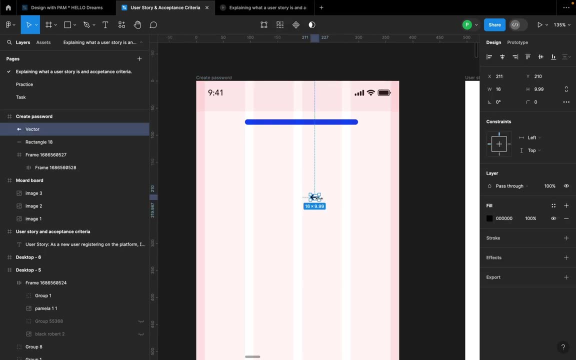 go to plugin and find hero icon. If this is your first time, just go to manage plugin and type hero icon here And you can find, click on it and then use that icon. But I already have it copied on my clipboard So I'm going to paste it here. 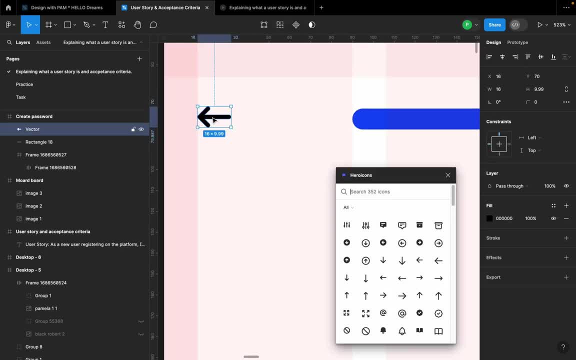 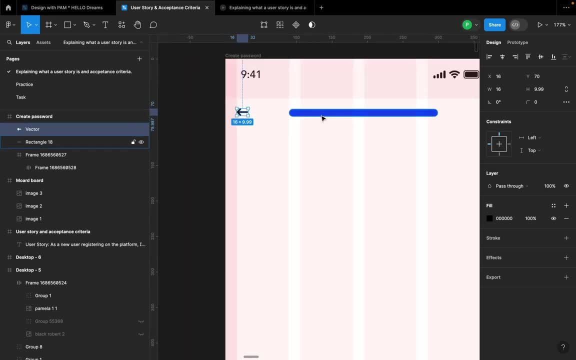 I'm just going to bring it here and make sure that it is aligned properly here. So this is the hero icon. You can find this icon, any of these icons here. use any of the icons here. I'm going to select this too. 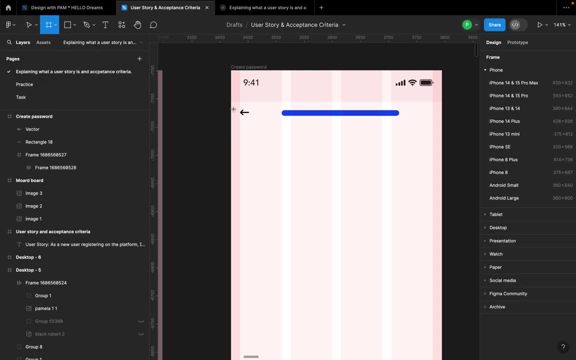 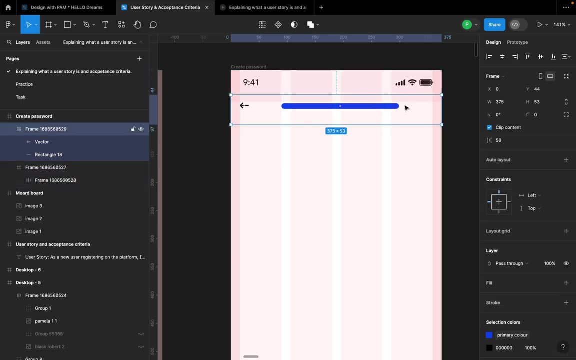 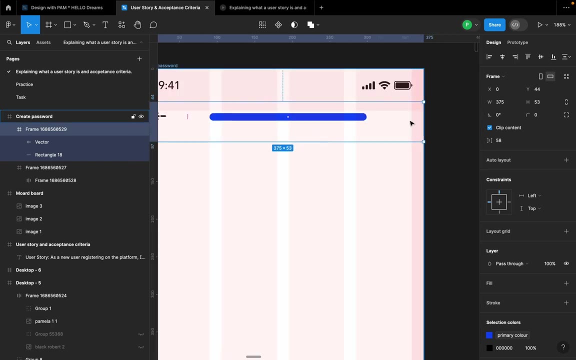 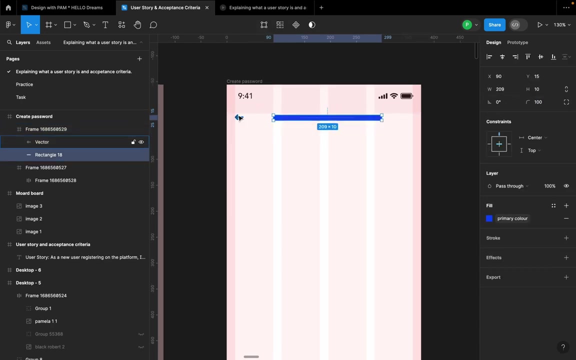 And okay, So let's just put it in a frame of his own too. Let's give it a frame. This frame is here. Let's put this one here For the frame here. let's make the frame height: Let's just make it a 50, then let's make this an auto layout. 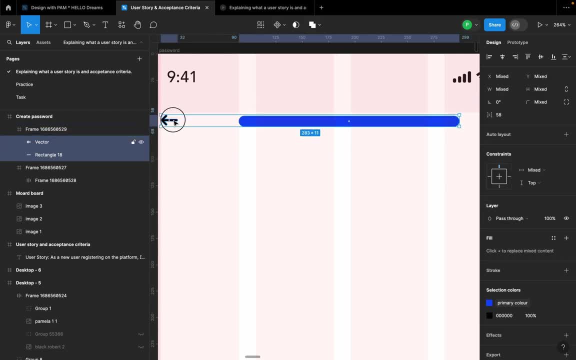 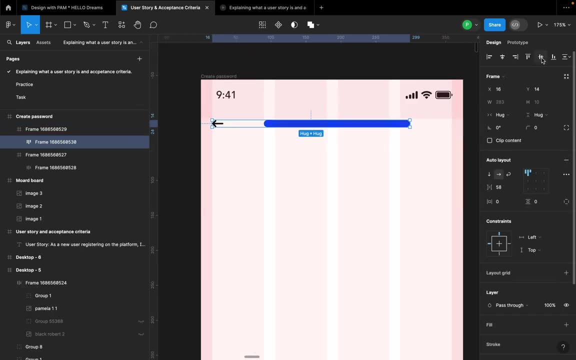 I'm selecting. I'm clicking this one, Then I'm clicking the second one by holding on to shift. Then I'm going to click shift a to create an auto layout. I'm going to make sure this is aligned vertically, So it's somewhere in the middle. 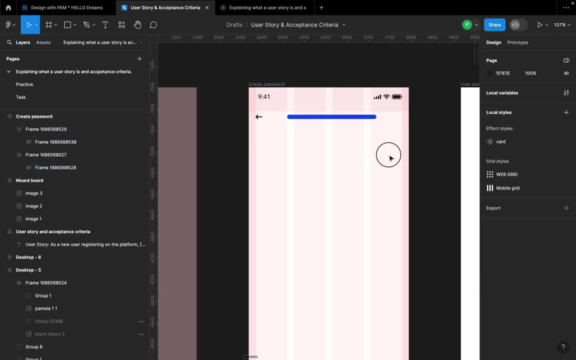 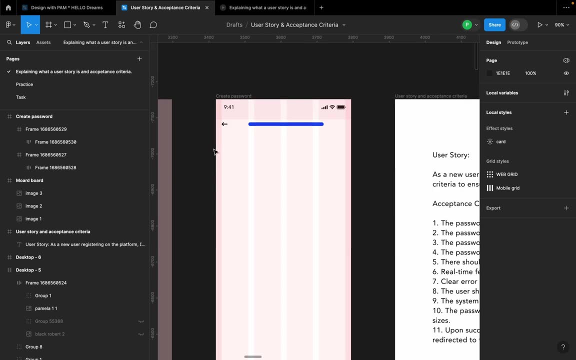 This is good. So, after creating this frame here, the next thing I'm going to do is create the title of the page, which is create password. right, We're dealing with create password. So I'm going to type T on my keyboard and I'm going to type create a password. 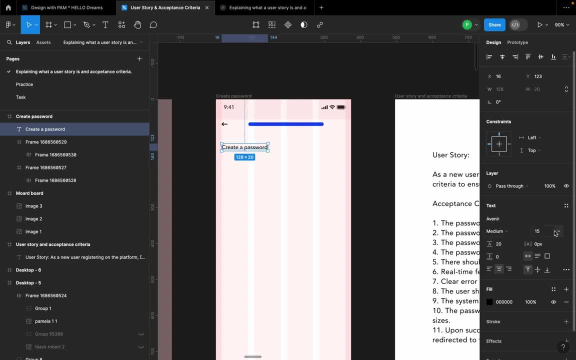 I'm going to make sure this is here. So let's make this font. Let's make it a 24. And let's increase it to a heavy, but let's change the color. Let's make this color 1e1e1e. 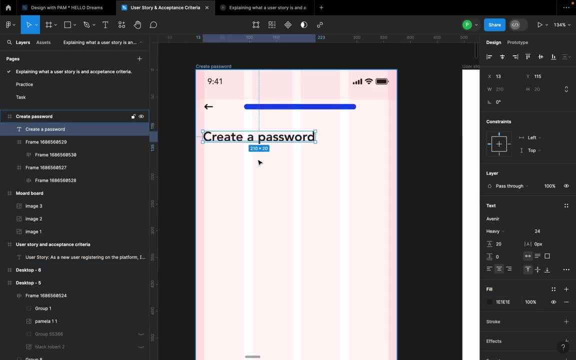 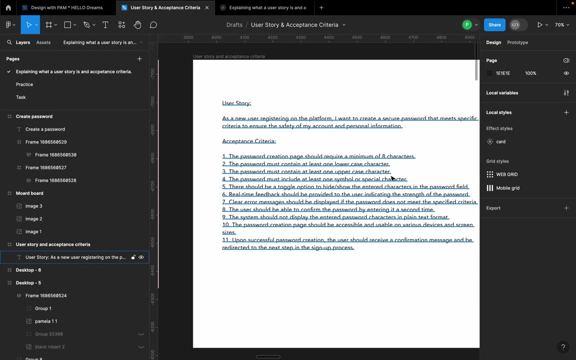 I don't want it to be To be as dark, So let's change this font to DM Serif Sans. This is good, So the next thing we're going to type is a test, right? So remember that. he's telling us we need to tell the client that there's. 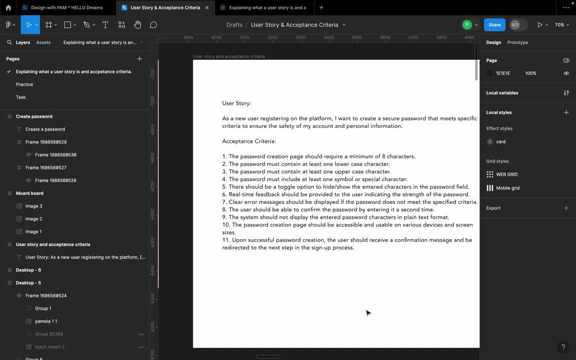 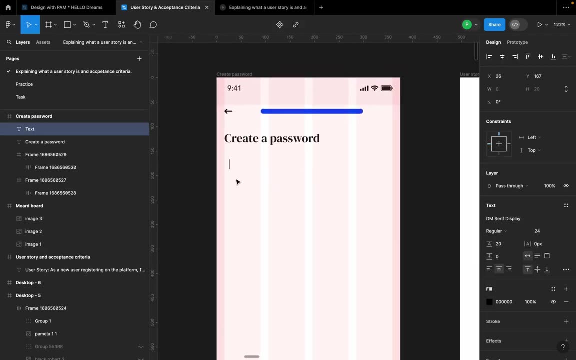 a criteria for the password and the need for creating the password right. So um says minimum of eight characters, um must contain uppercase and all of that. But again, let's just give this page is subtitle. I'm going to hit T on my keyboard and click on it. 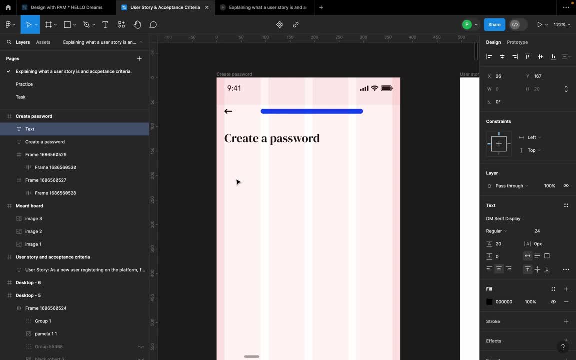 And I'm going to type, I'm going to see: um do we need? let's inform the client that they will need this password to assess their account. This password will be used to assess your account. So what I'm going to do is I'm going to reduce this font to up to 16, but 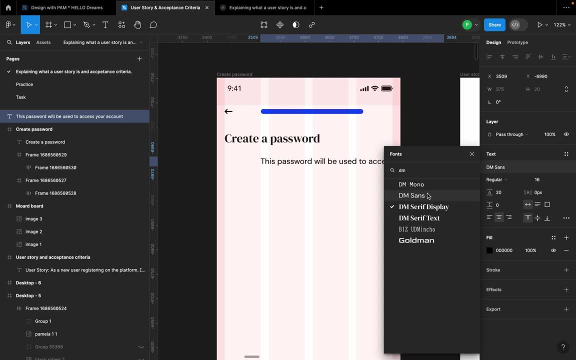 I'm not going to use DM Sans for this. Let's use DMS, just DM Sans, like this. Uh, let's reduce this and let's make sure that it is left aligned like this, But again, let's reduce this to a 14.. 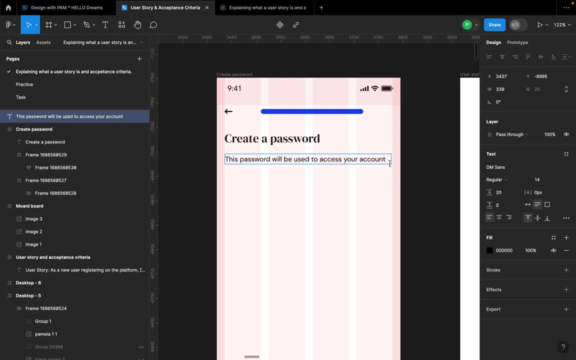 Then I'm going to increase this like this: So this password will be used to assess your account. Password must contain: must contain lists, eight characters long, and contain a mix of of upper and lower case, lower case letters- lower case, I think- numbers and 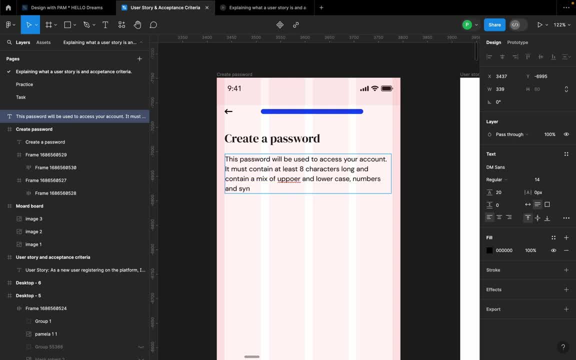 symbols. So let's right click on this. This is okay, but let's see if we can. I think 20 is okay. Let's see if maybe let's use this and for this section again, Let's use this so that this is properly aligned. 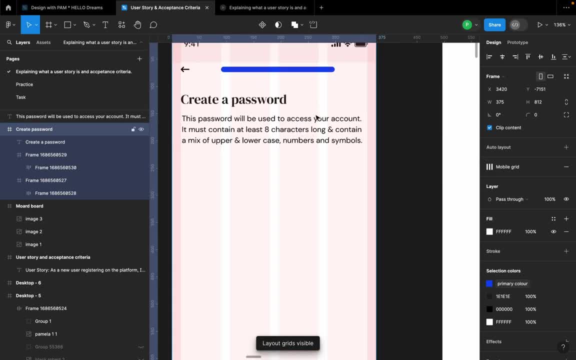 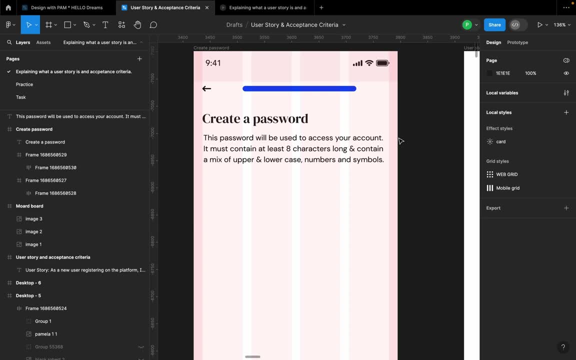 This is okay. This is okay. Um, one thing I want you to know is that you need to create some form of hierarchy when you're making your designs. So this one is on black. Um, I'm using the shade of black and it's quite bold. 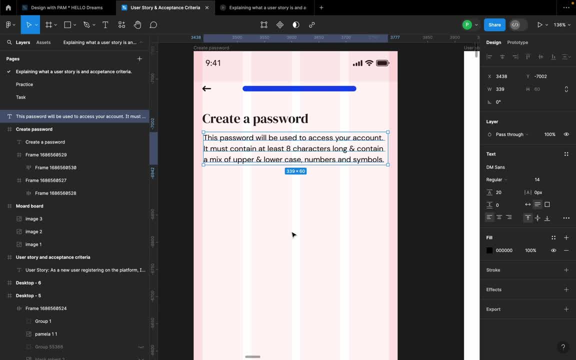 This other one appears strong too, So I'm going to give it a different color, so that it's not going to be competing for attention with this particular one, because I want you to notice the title. The title comes first, then the subtest second. 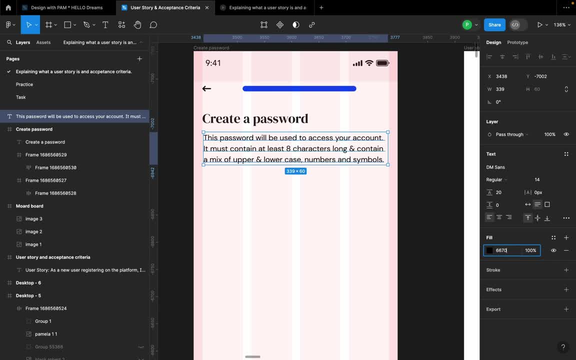 Well, I'm going to give it this color code: 6670885.. This is better. What I'm going to now, though, it's select this one, hold on to shift, select the other one and create an auto layout. I don't think I did that properly. 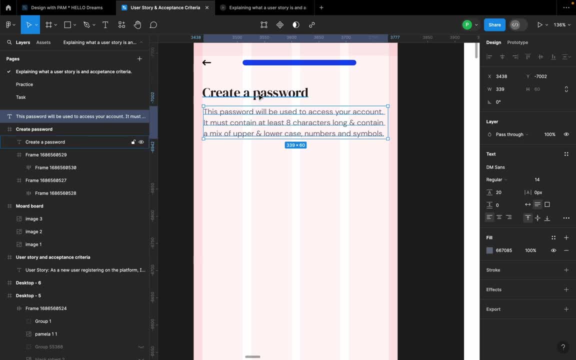 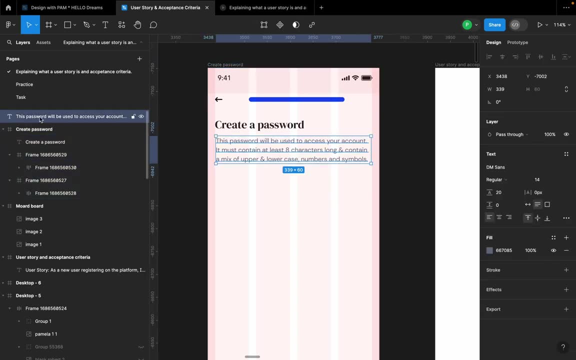 Okay, So, as you can see, when I did this, it didn't quite work very well. That means this: This one is not inside the parent frame, which is this frame that we have here, This one. look at it here. 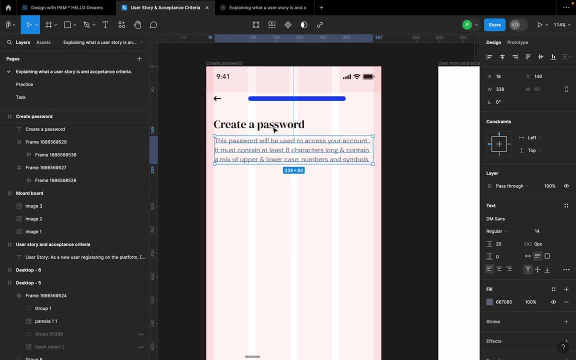 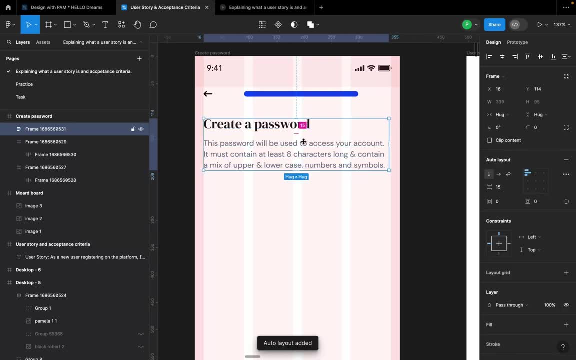 If you look on your left hand side. I'm just going to bring it in, So I'm going to select the first one, select the second one and create an auto layout by hitting shift a for the space in here. we can give it between 12 and. 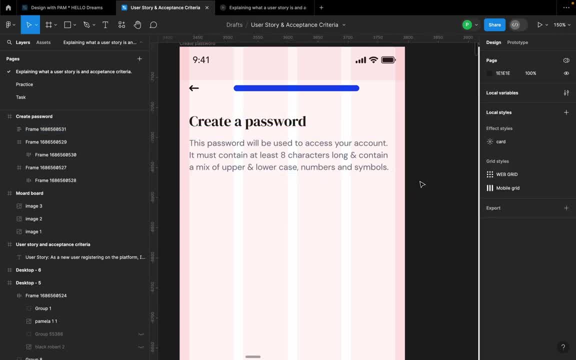 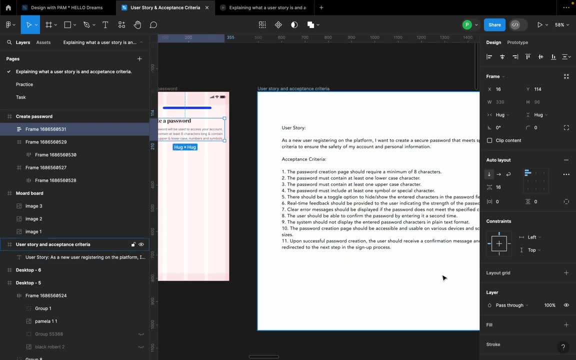 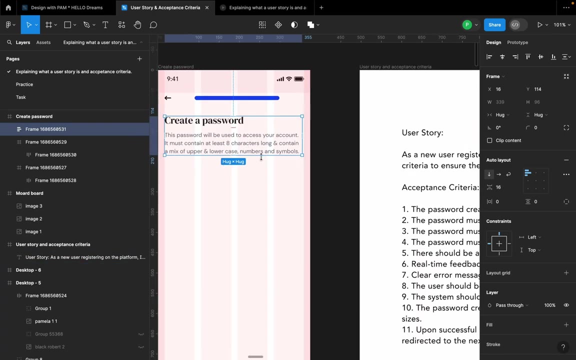 maybe 16,. let's try 16,. 16 is good. The next item we're going to do now. we've created a title and somehow we've hinted them about the requirements: Number of characters, lower case um, lower case, numbers and symbols. 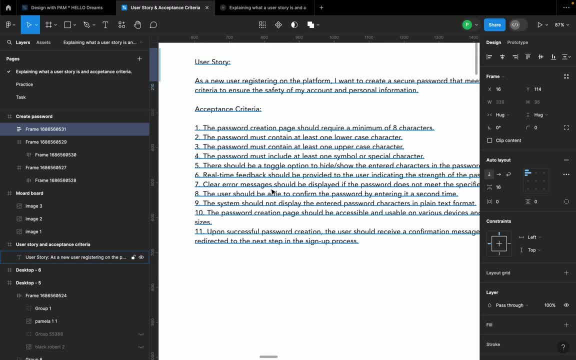 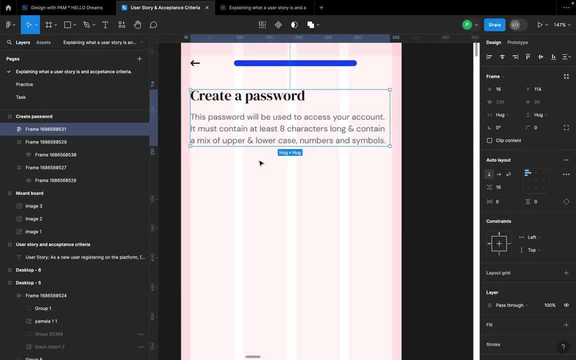 However, there's another portion that says that real time feedback should be provided to the user indicating the strength of the password. So we're going to do that, but let's create the password field like input field, where user will provide the password itself. 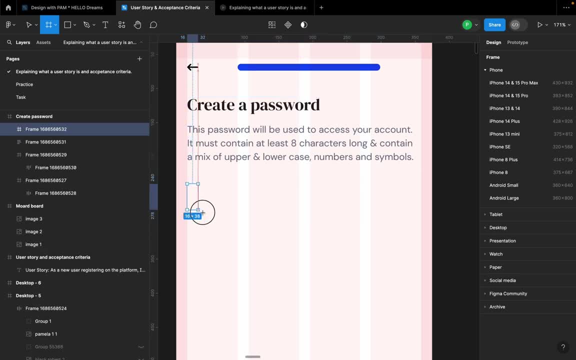 Let's do. let's use a frame here. I'm going to click F on my keyboard And I'm going to draw a frame. So for this frame, I'm going to give it a height of 44,, which is good. 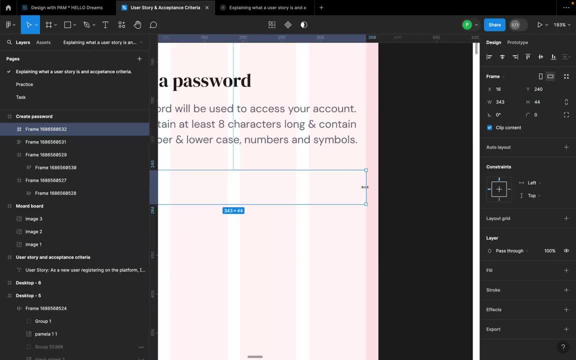 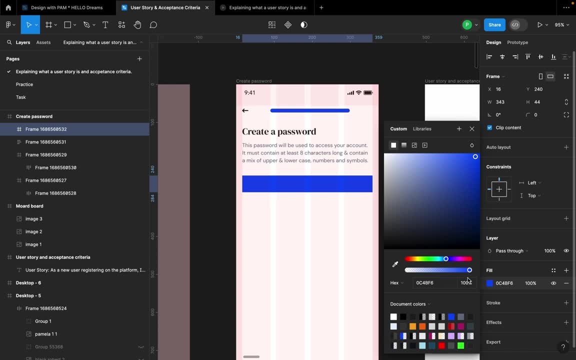 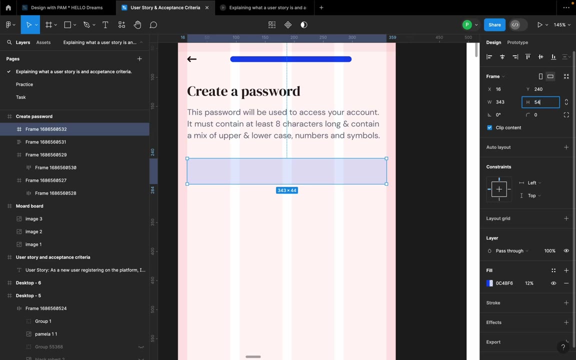 Make sure this is aligned to our grid lines here. Now, let's give it a few color. Let's use this, our primary color, blue. However, let's reduce the opacity very well. Now we should increase this. let's increase this to a 54.. 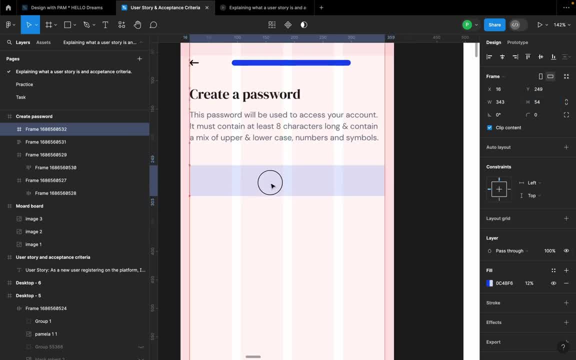 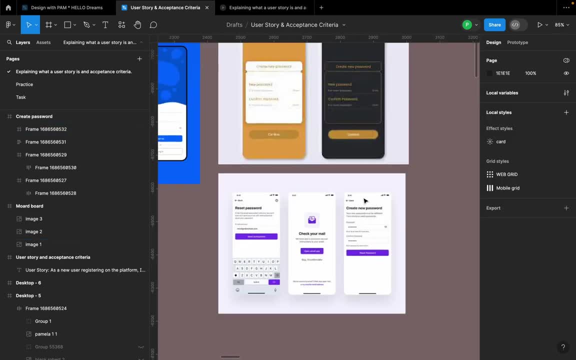 This is better. I'm going to bring it down a bit. Let's give it a corner radius of. let's give it four, Right? So let's do that. So what we're going to do is remember we have this, some sort of thing. 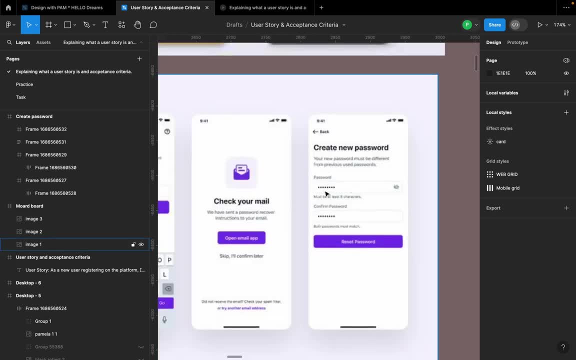 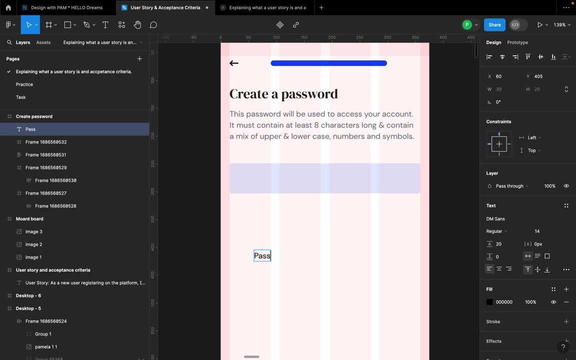 Maybe we should go with this um a header, then a section here, So we have um. let's click T on our keyboard and type password. I'm going to bring this two down a bit, So for this one I'm going to make it a 16.. 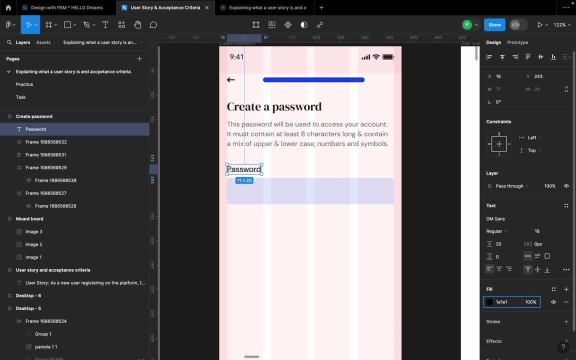 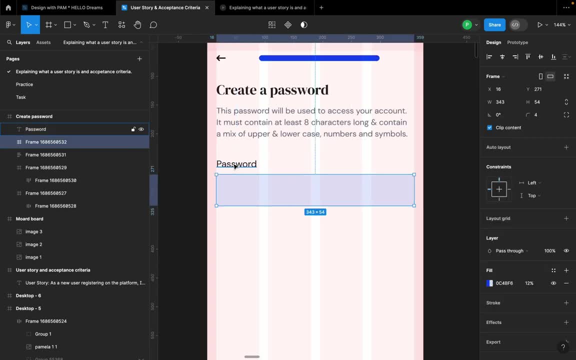 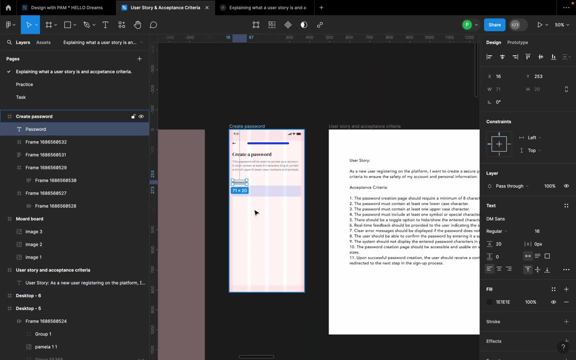 But let's change the color to one a, one E. let's leave it, that's no, let's leave it, That's right. So the next thing I'm going to do is to create this section here, This thing that says the system should number nine. the system should not. 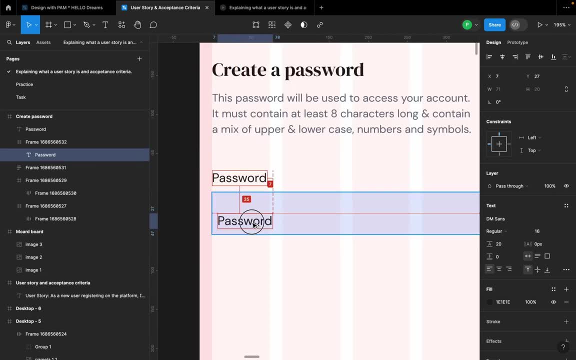 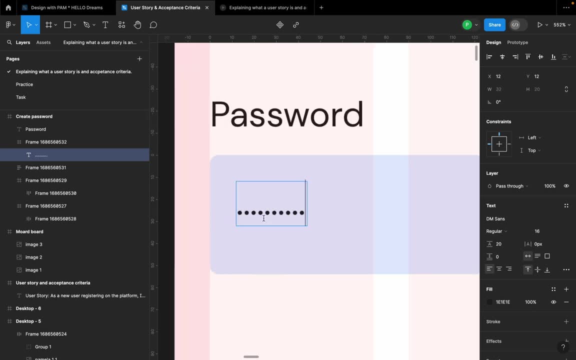 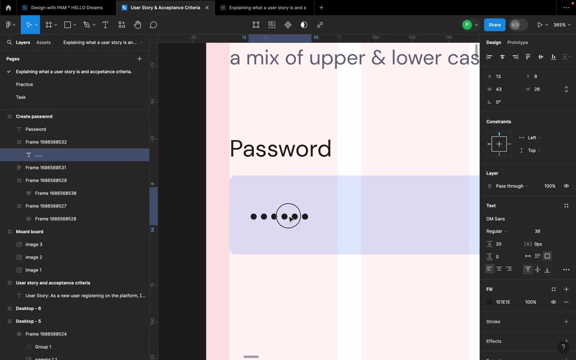 display the entire password characters in plain test. So I can either do this. Password characters. Let me see, I'm going to increase it to 36.. It's fine, I'm leaving you here. So this is more like an indicator. 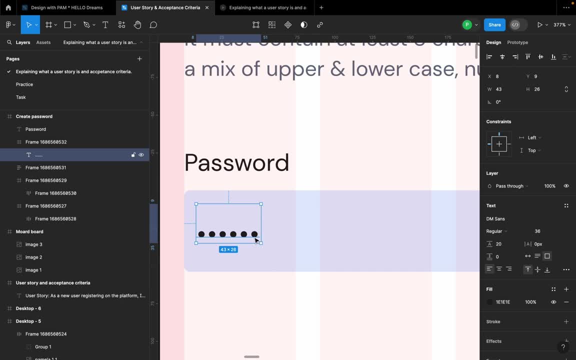 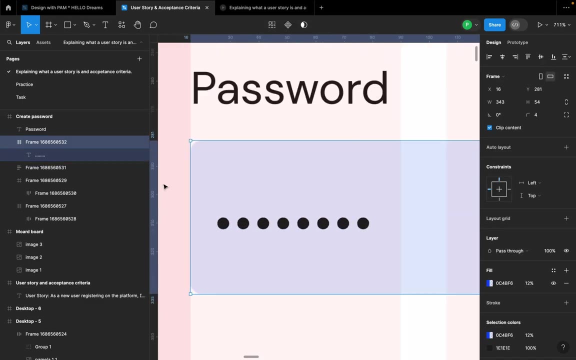 So he said it must contain at least eight characters. so let's see, let me increase this a bit- two, four, six, eight. so maybe this will serve as an indicator when you're punching your password and this is what you get to see. or maybe, when you open the toggle, the 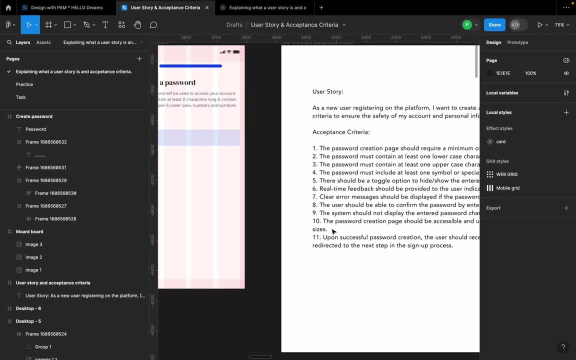 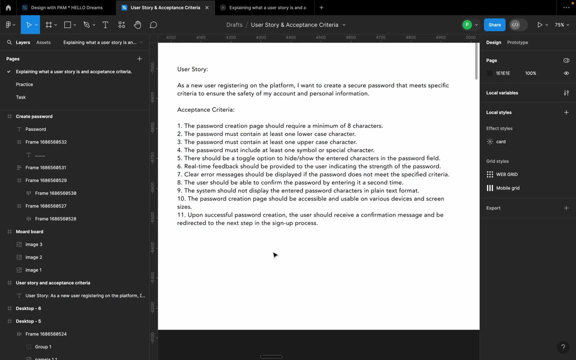 eye toggle you get to see your the password that you have imputed right. so you remember that there's an acceptance criteria here that says number five. there should be a toggle option to hide slash, show the entered car attacks in the password field. so i'm going to right click and go to hero icons here. 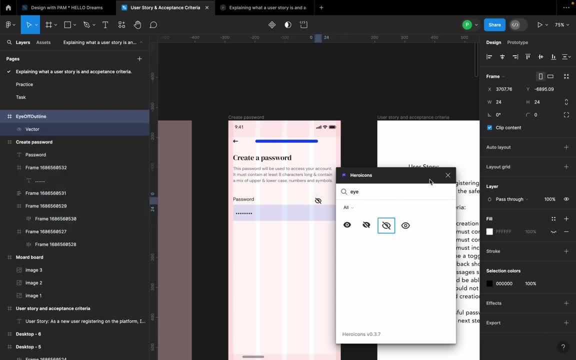 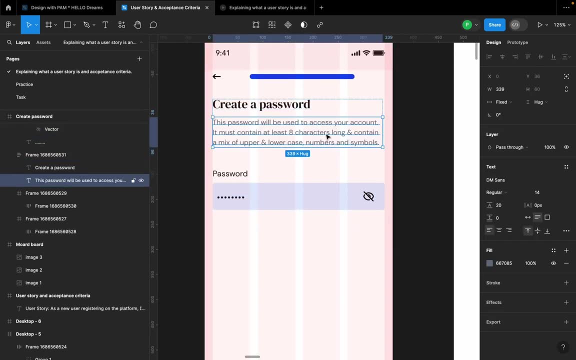 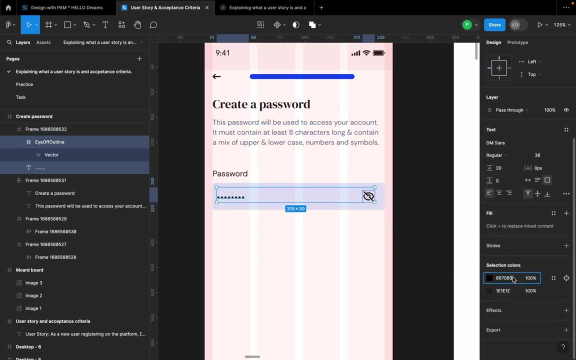 then i'm going to find an eye. i think this is fine. i'm going to bring it into the frame here, but what i'm going to do is i want to use this color, this color here that i've been using here, because i don't want it to be too dark. i'm going to select the two and make sure i change the color. 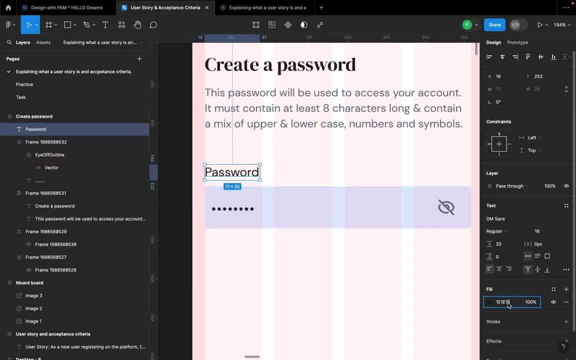 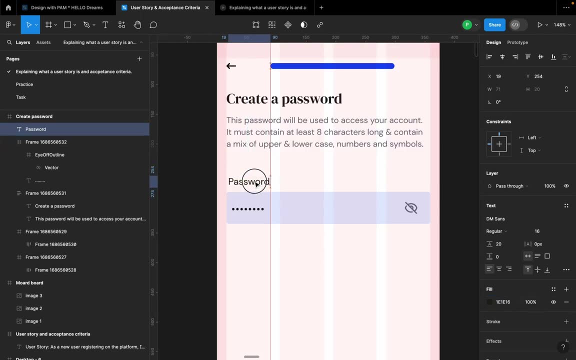 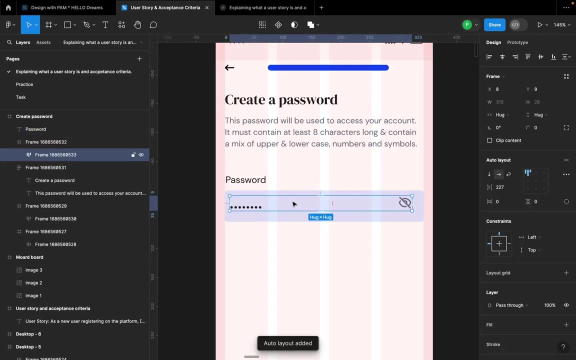 to that. so this one, maybe we should change the color to this one too, make sure it's on 100, and i think we're good. so let's select. i'm going to select this one, select this to make it an auto layout, and i'm going to make sure that it is centered here, and i'm going to come to this. 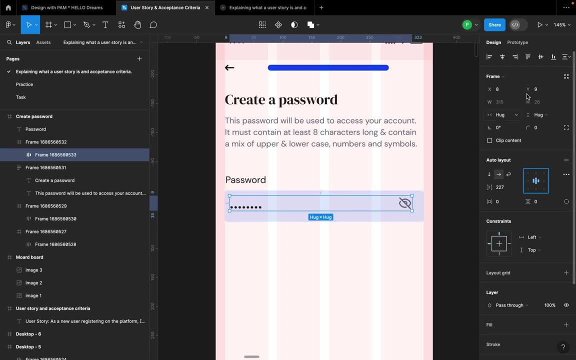 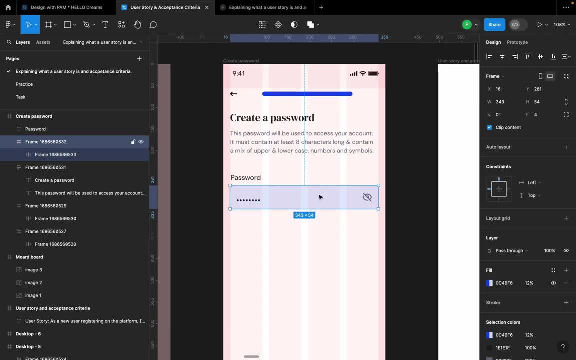 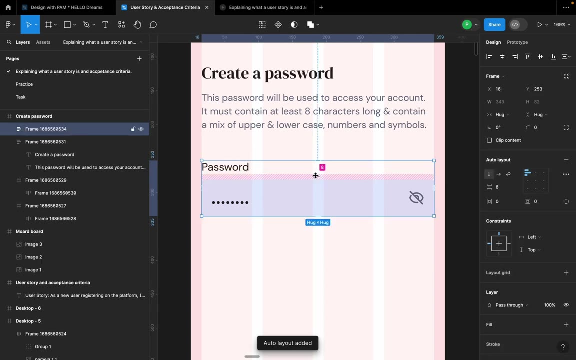 place to make sure it is centered also to the parent frame. so i'm going to click on this vertical alignment and also this. so next thing i'm going to do is i'm going to select this, select this first one and also create an auto layout. the spacing in between this one and this one is eight, which is: 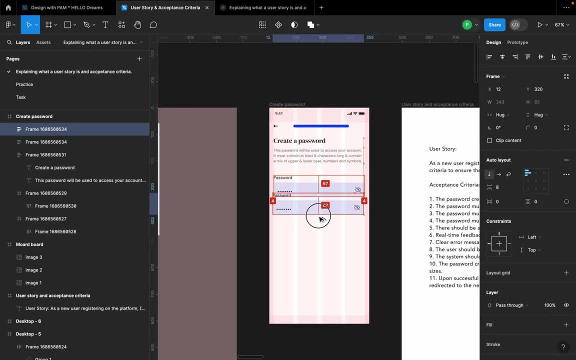 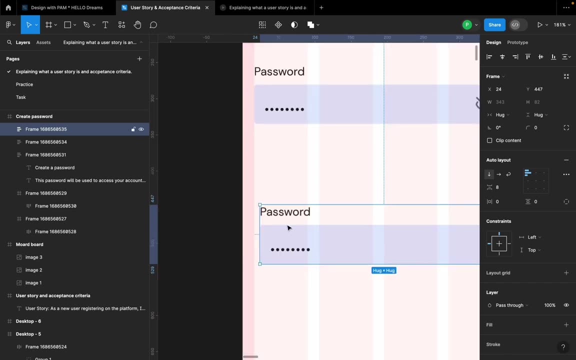 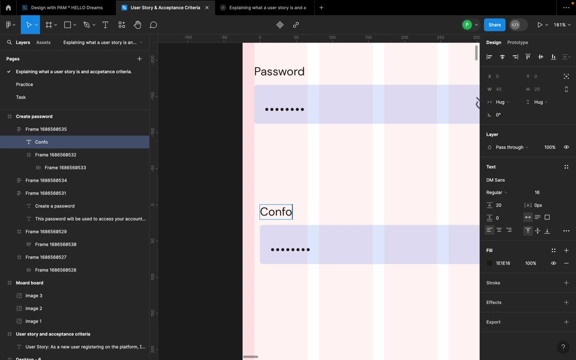 good, so let's go ahead and duplicate this. i'm holding on to optional alt key and i'm dragging down out with my mouse and i'm going to release my hand from the option and alt from my option, or alt and my mouse all at once. so this one, i'm going to say confirm password. 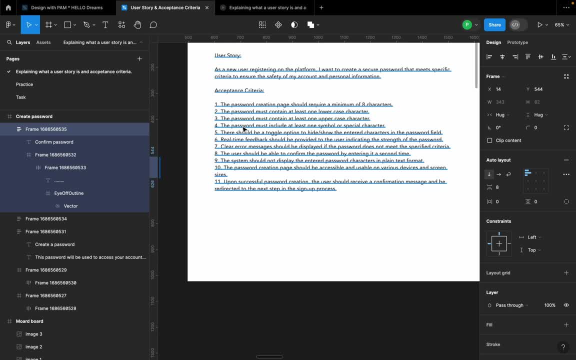 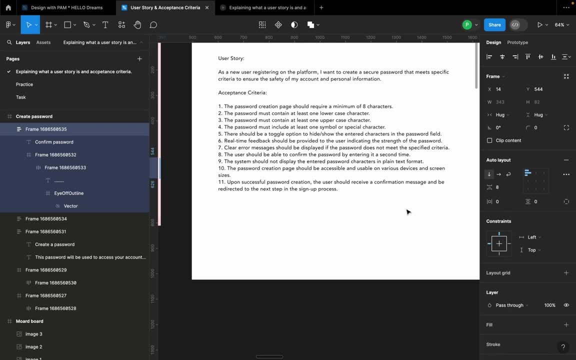 this other section, this number one, two, three, four, and i'm going to like spell it out clearly for the user so that they know that these are the requirements, and also remember that number six says that it should be a real-time feedback that should indicate to a user um that they have met the criteria um of the password strength. so 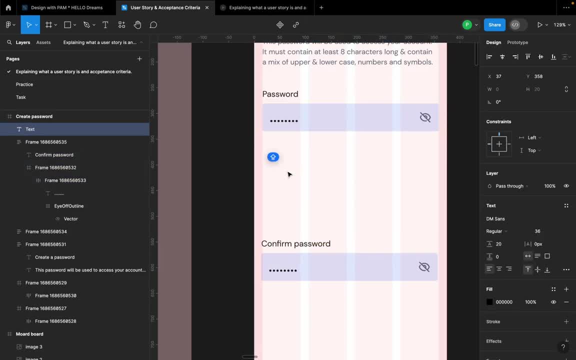 what i'm going to do is i'm going to hit c on my keyboard and i'm going to type minimum minimum, minimum minimum of characters. i'm going to reduce this font to right. so let's also this black color. let's use this color. 1e. 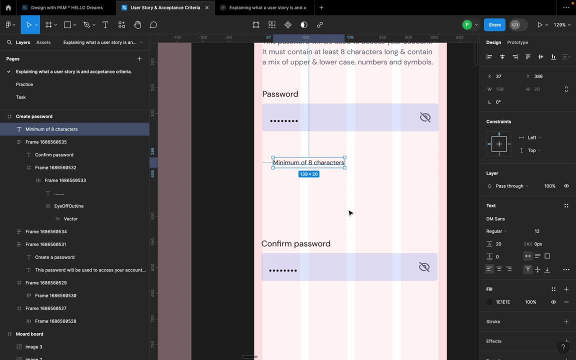 1e. so most times when we're designing, i know it's very tempting to use shouting colors and but you should always try to imitate a real life mobile application. so in as much as you've gone to dribble and you've seen very fancy applications or very fancy. 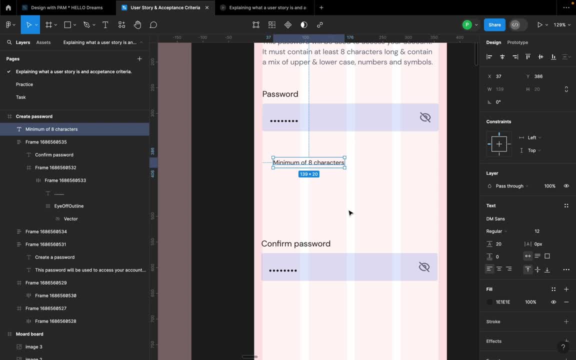 designs. try to mirror or design what is, upon it, obtainable on real life applications. so go ahead, download applications that are maybe speaking to what you're designing for. it could be a financial application or crypto application. try to onboard, try to see the experience again and get some. 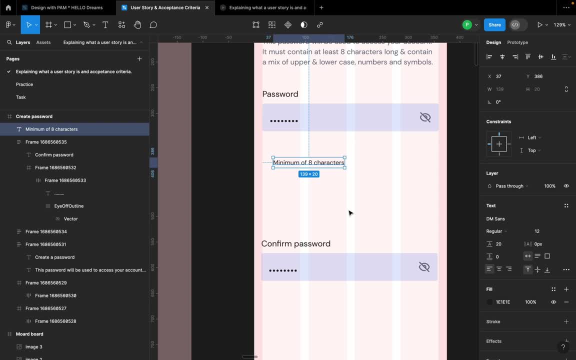 inspiration from this so you can design something that people can actually use and not something that is just pretty as a design. okay, so now we have minimum of eight characters. the next thing we have is at least one lower lower case letter. we also have at least one upper. other one is at: 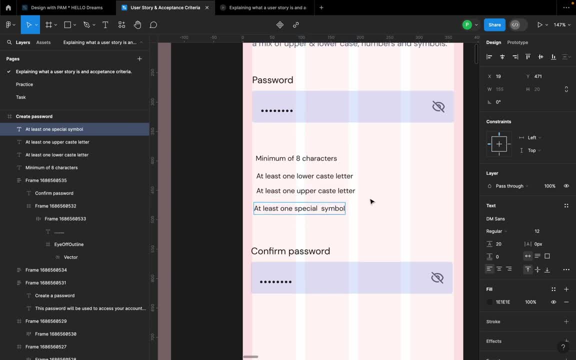 least one special symbol symbol. so sometimes i know that at the point there was a point where i used to be so confused on what special symbols are. so it would be nice if we also add some of this: special symbols for users. i don't think and add are at this, at this, at. 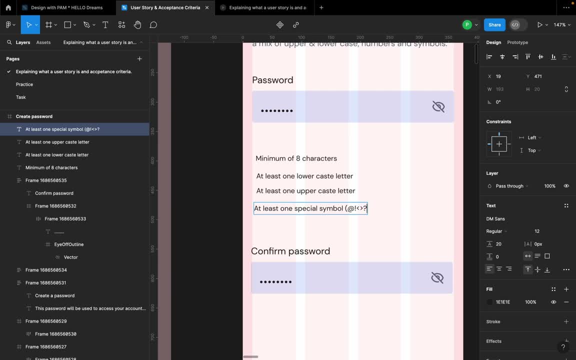 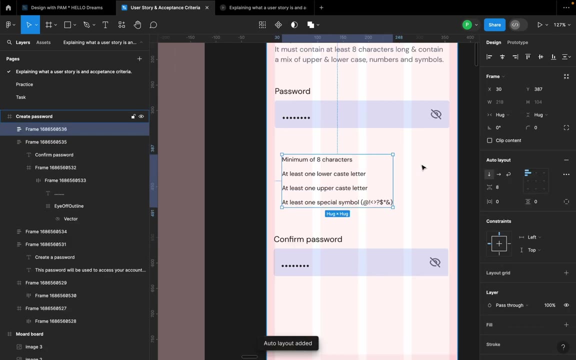 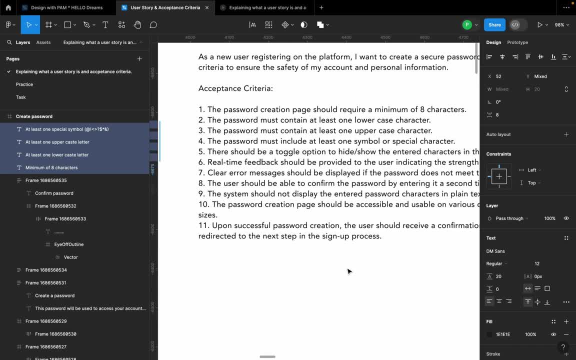 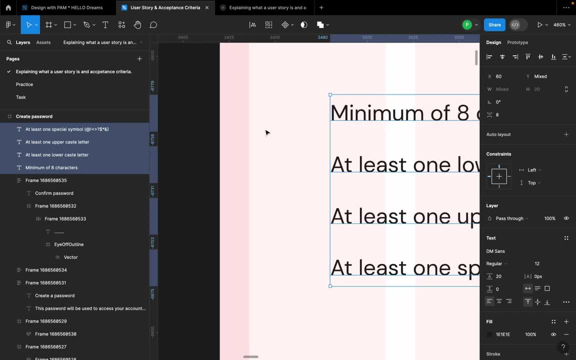 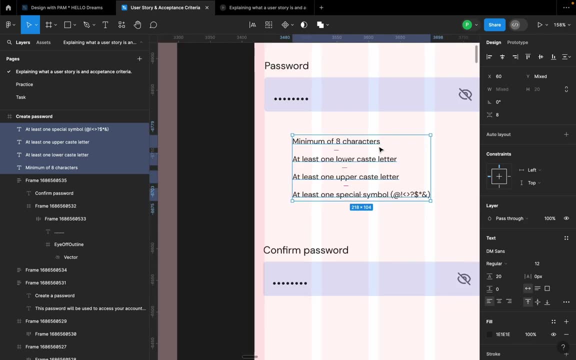 told that we should do in the acceptance criteria. we should um provide read time, um feedback to user. so i'm just going to click something like a checker. so, when you have entered maybe a minimum of eight characters, it's going to indicate that you have entered, uh, eight characters. so i'm going 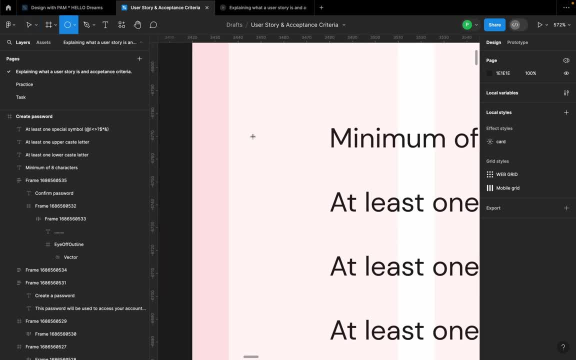 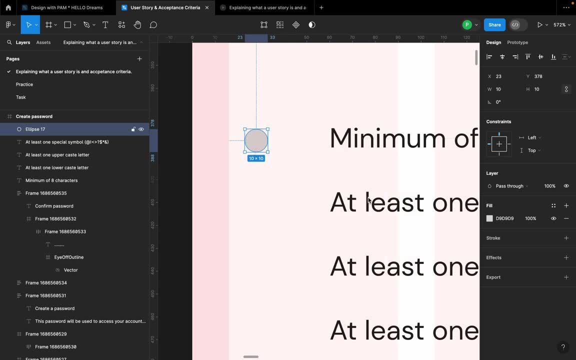 to click on, oh, on my keyboard and i'm just going to draw a a small cycle here. so i'm going to right click, go to plugin, go to hero icon. i am going to find a check mark here. i'm going to bring this one in. i'm going to remove this from the frame, delete this. i'm going to hold on to. 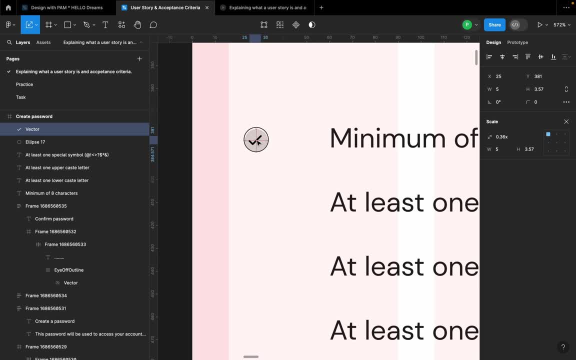 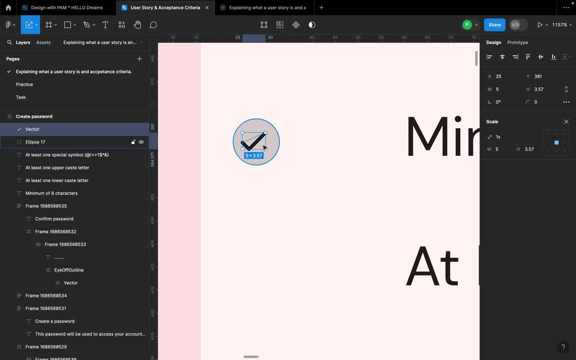 shift on my keyboard and i'm going to add it here, so make sure this is aligned. so i'm going to select this icon, hold on to shift, select the cycle that i created and right click on my mouse and group the selection here. so remember, um, i'm going to go back and click v on my keyboard to go back. 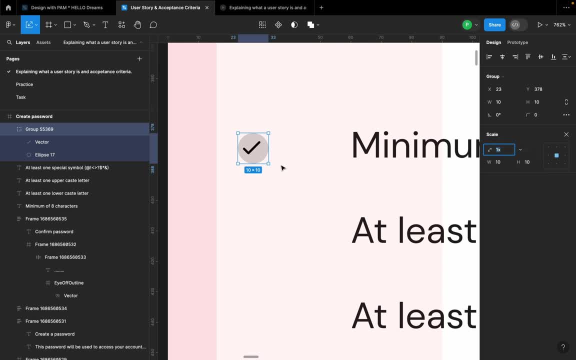 here because it was on skill and activate a skill by clicking k on my keyboard so that i can scale something right. so i'm clicking now command z or control z to go back to my initial position and i'm going to click on v on my keyboard to be on my move tool. so remember that we have to also maintain. 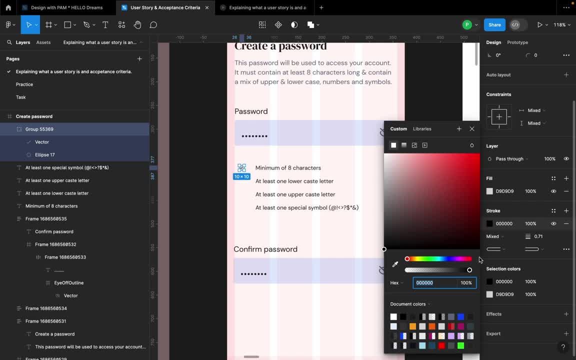 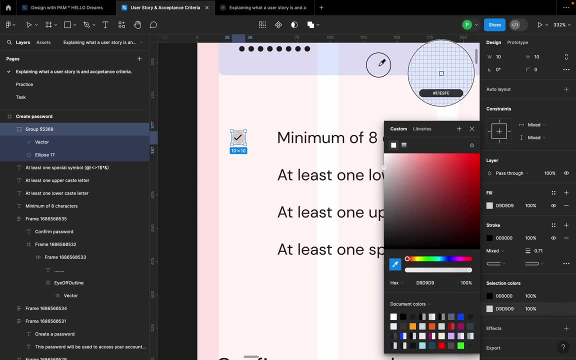 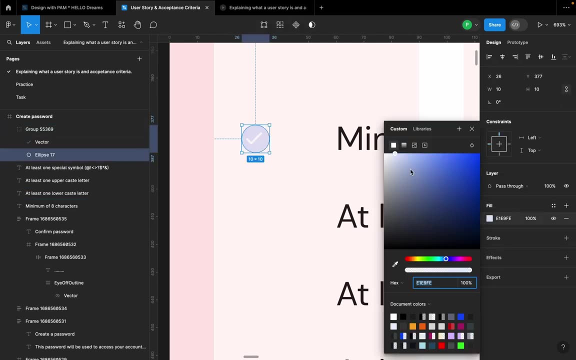 a same color, right? so i'm going to try as much as possible to make sure that this ellipse here has a color, the color that we're using. this one, i'm going to change it to this particular color. then this one, let's make it in white, and this other one, let's try to darken the color just a little bit. 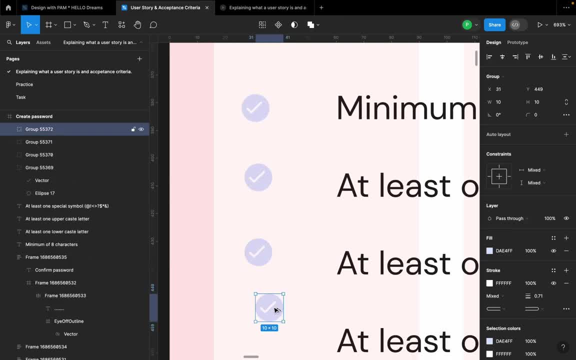 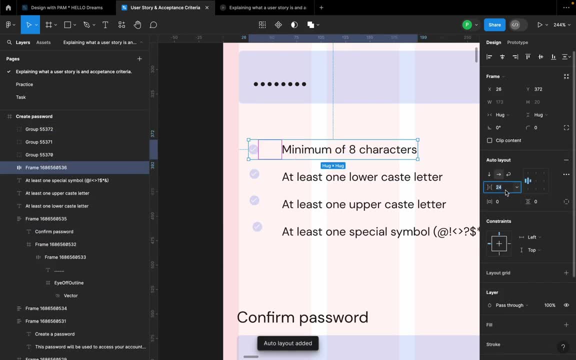 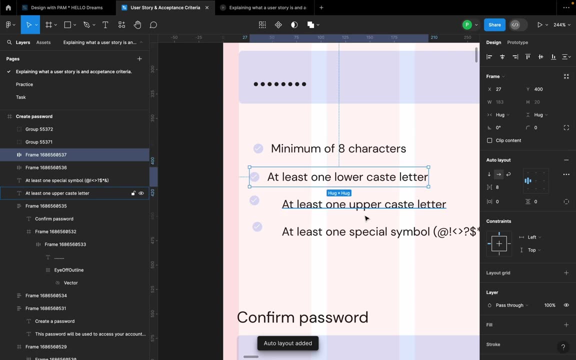 all right, so i'm going to duplicate them into four places. now i'm going to select this one. select this one: hit shift a to create an auto layout. make sure the spacing between it is just eight. here i'm going to do the same for all of it: make sure the spacing is just eight. 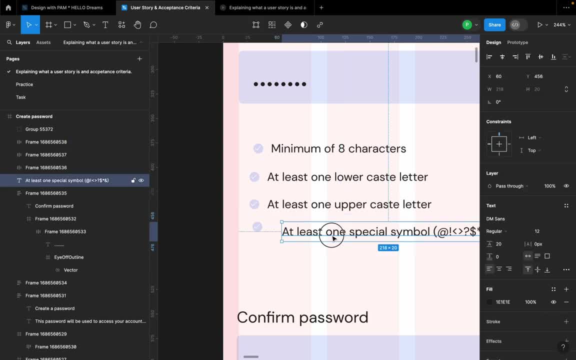 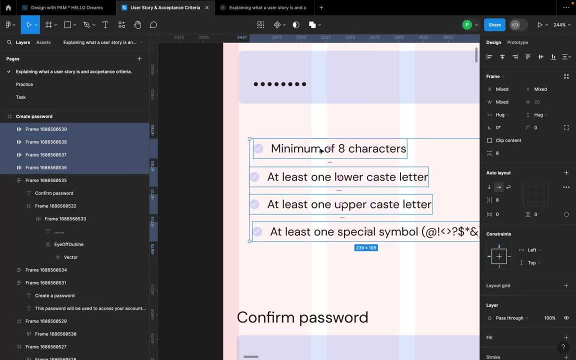 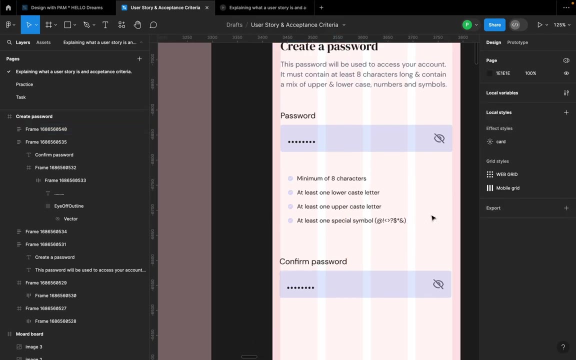 make sure this is aligned here, make sure the spacing is eight. i'm just adding an auto layout in each of them. then i'm going to select each of them- this first one, this one, this one, this one- and create an auto layout here. now. this is going to be an indicator, but i wouldn't want to just leave it like that. 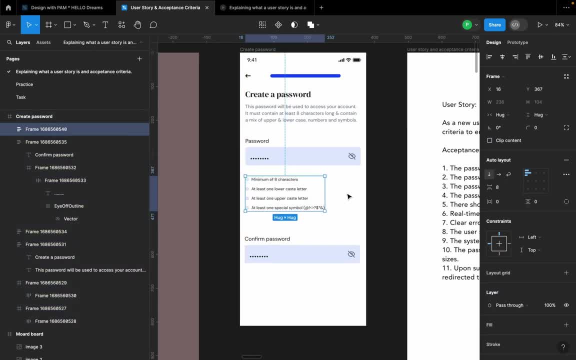 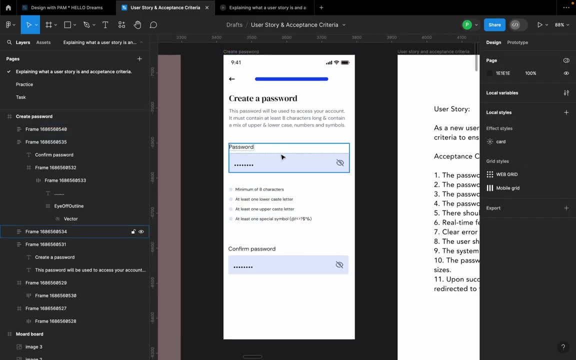 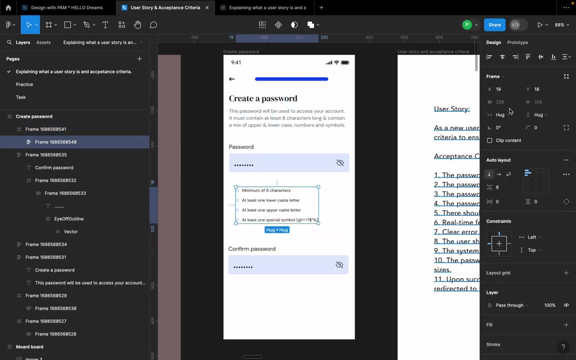 let's close this mouse, so you can try to leave it like this. however, it might not be that appealing to the eyes, right? so let's click on f on our keyboard and just add a bit of frame around it. i'm going to shift this here. make sure that. so let's align this in the middle here to this frame. 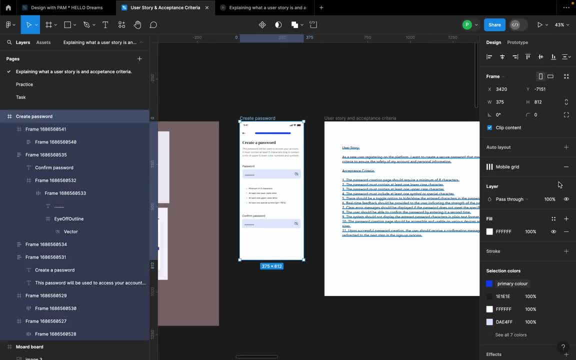 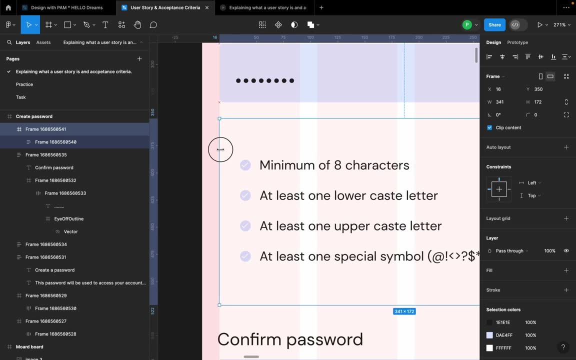 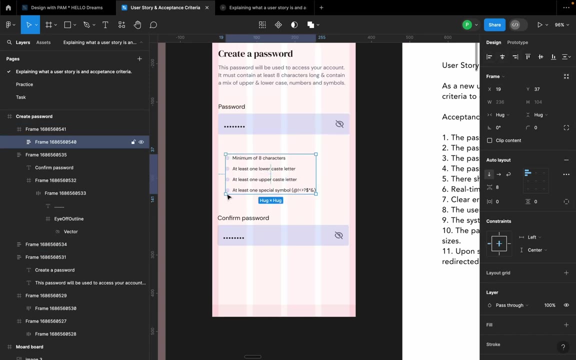 now, let me give the frame a height. let's put back our grid line. so we see what we're doing. we make it here. make sure that it goes on our grid line now. let's make sure the spacing between this, however, so so that you can see the frame itself. 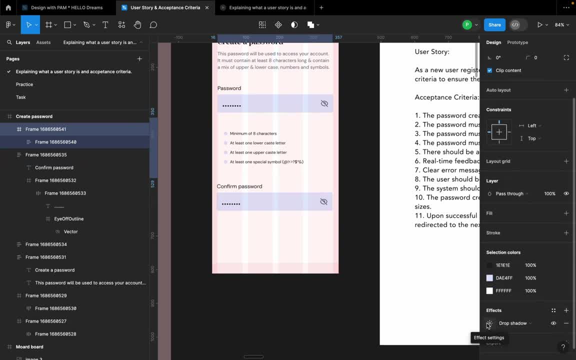 right, i'm going to add a bit of an effect here, just a little bit of drop shadow. so for this drop shadow, let's give it a color of one zero, one, eight, two, eight, right. so for the x section, let's leave it at zero, the blur let's make it a six. the y section, let's make it a minus one. 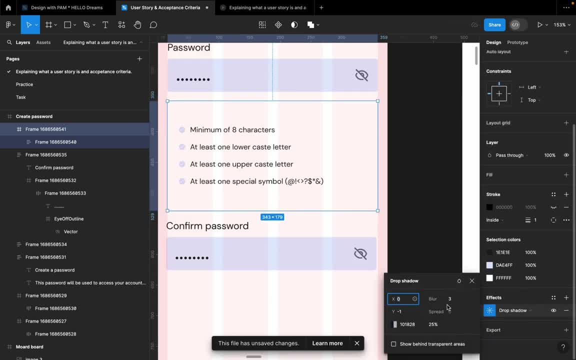 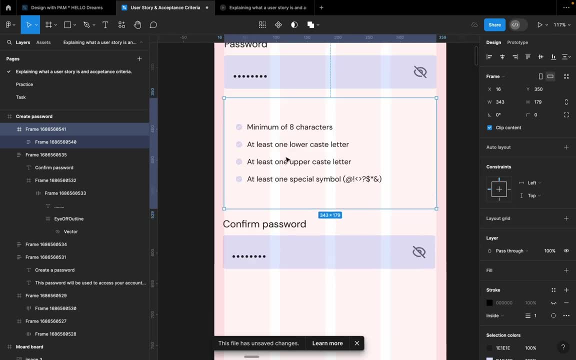 right, all right. so after adding this, um, this effect. so let's keep this at three and this one is 25. this is okay. what we're going to do is make sure that we add a field to it so we can see what we're doing, and let's try to change the corner radius to um an eight and it is good, all right. 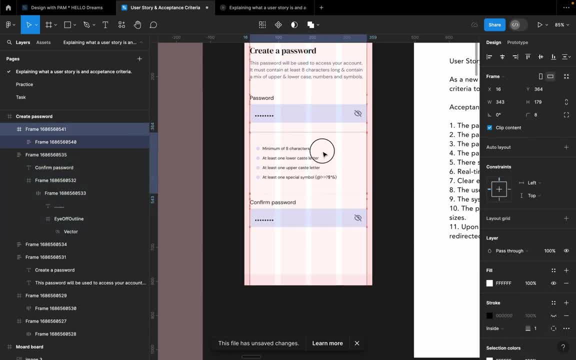 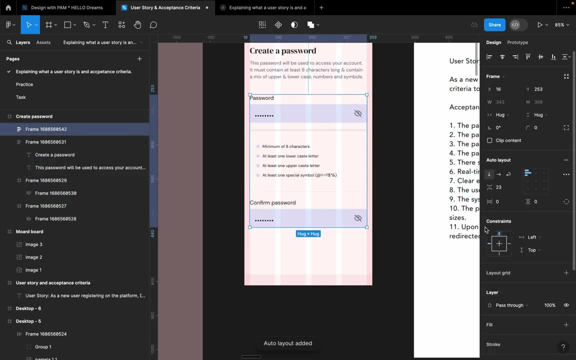 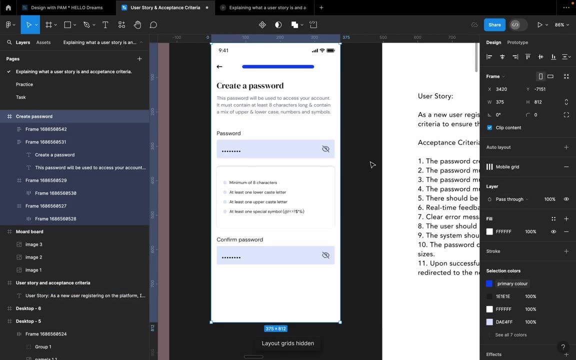 so this is fine. so let's try to align the spacing here, the spacing between each of them. i'm going to make sure that the spacing between them is 24, which is fine. so if we hide our grid lines, now, this is what we have going on here, but we can go ahead and try to reduce this opacity to. 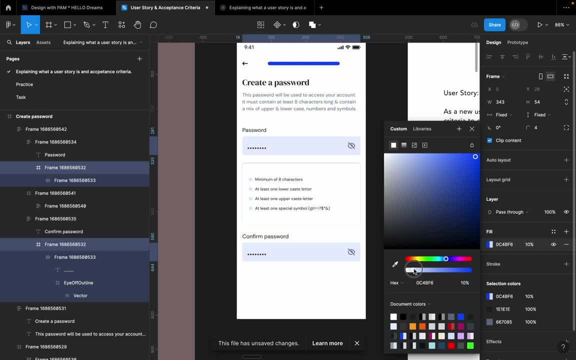 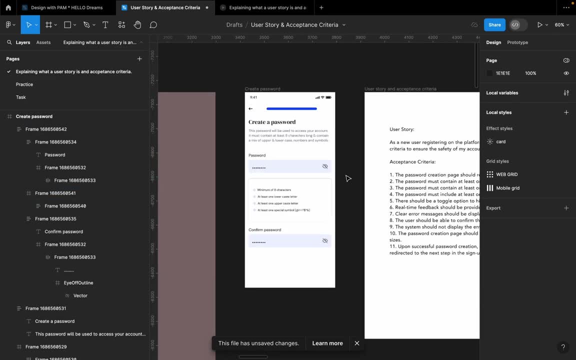 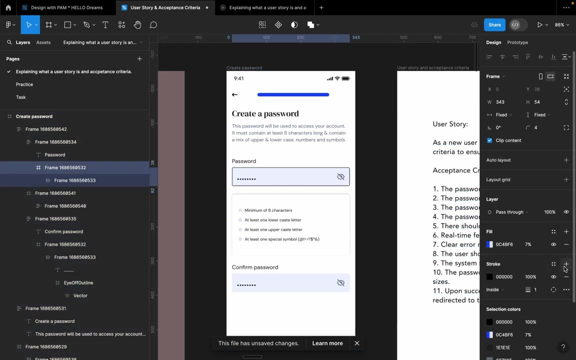 just a little bit again because i don't want it to be too shouting. now. if you notice, here i use very calm colors and i'm not like being too dramatic here, like making, let's imagine, i made this, i gave this a stroke, maybe gave it even a blue color, because the 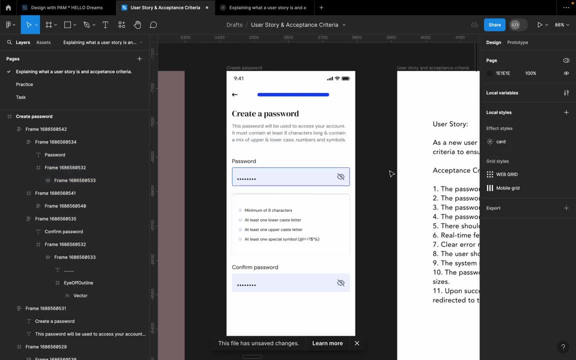 company says that they're blue. it doesn't really make it look very, very professional. when we stick to colors that are calm, all right. it just tends to make it look as if um, like a serious professional, has designed that um screen that we're looking at. so the next thing we're going to 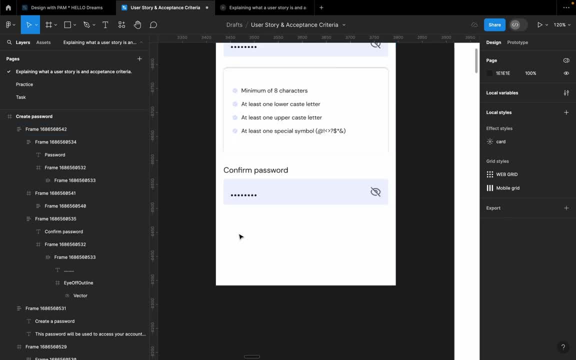 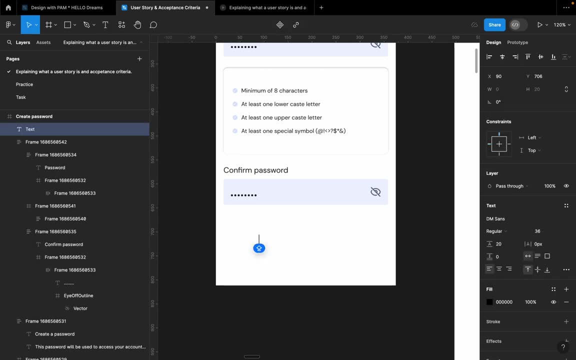 do now is to create our call to action button. so what i'm going to do is just to click t on my keyboard and i'm going to say: what are we going to title it now? should we say okay, let's just say continue. so, but for this one, i'm going to reduce the font to let's leave it at 20.. 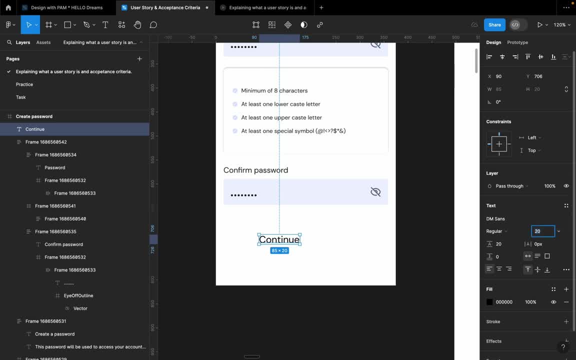 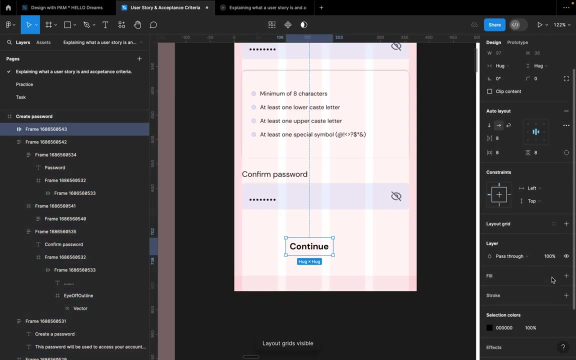 now let's make it an 18. 18 is fine, so let's also make this bold. so i'm going to hit shift a on my keyboard. make it a, not a layout. what i'm going to do is i'm going to put back my grid line on and i'm going to give this a fill. make sure the call to action button. 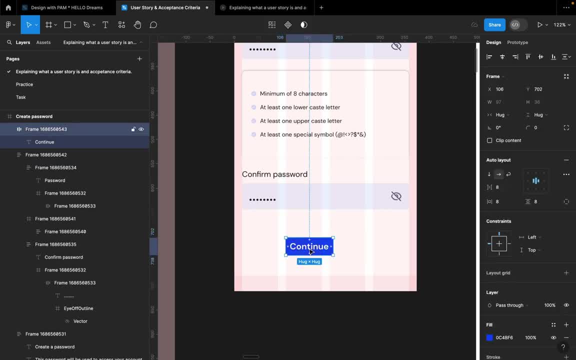 is in blue, so i'm going to make this white. you can see, from black to white it looks better off. i'm just going to increase this here. let's give the corner radios a 4.. make sure the height of this card is a 44. 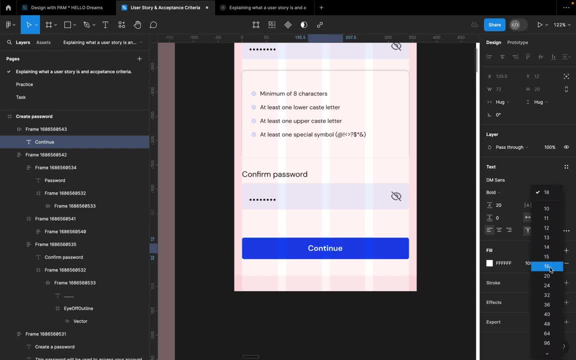 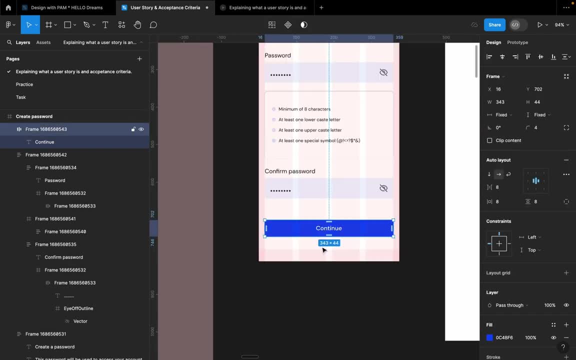 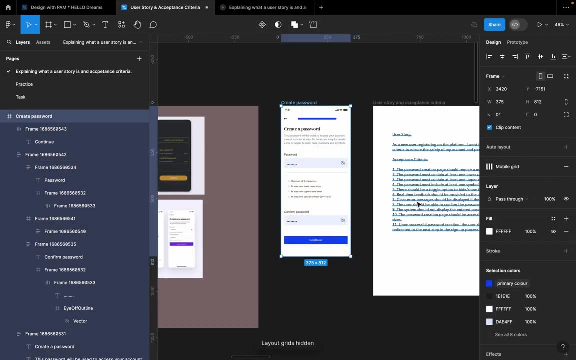 which is good. let's reduce this to a 1.8 inch 16. let's make it a medium. so this is good. make sure the space in between this 250. it is okay now we have created this card here. we have created this card here. 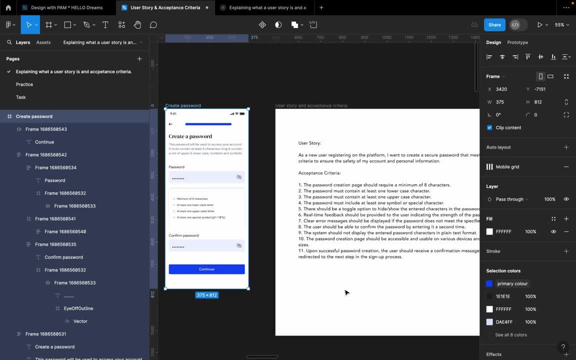 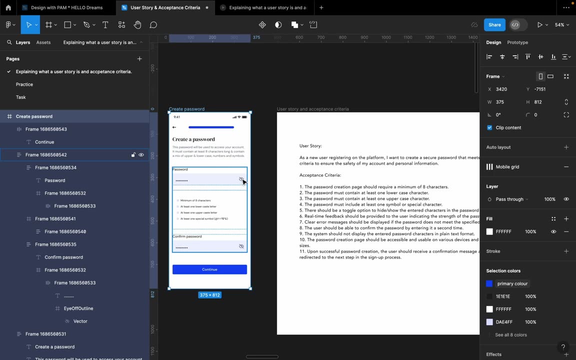 that's refused most of the criteria if he feels one, two, three, four and also fulfills five right. we've told the clients, giving the client of this information, and we've reviewed five, which says there should be a toggle option to hide or should enter characters and a password, which is this: 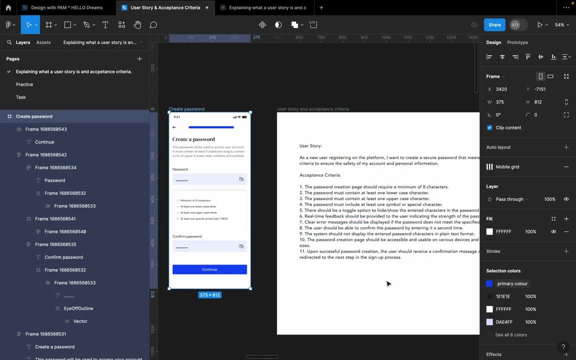 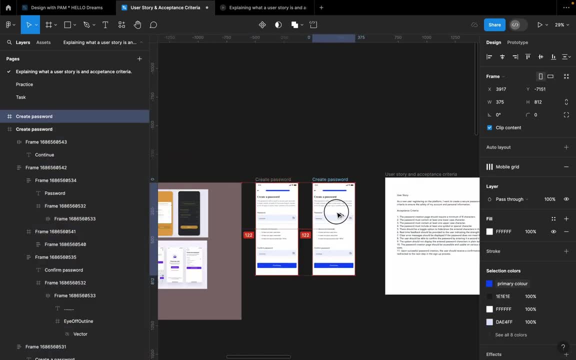 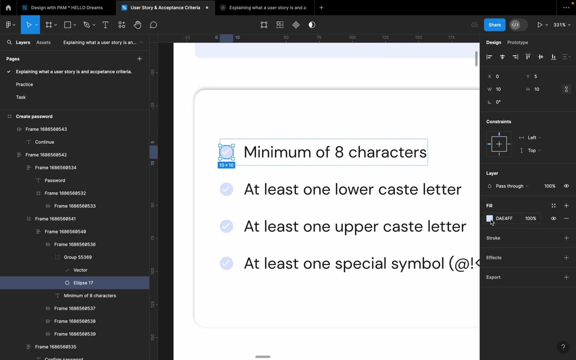 eye icon here read time. feedback should be provided to users indicating the strength of the password. now this is what I'm going to use achieve that particular user story. so at this point, remember, I put the check right here. so when a user has refused this particular criteria, this check should turn green. 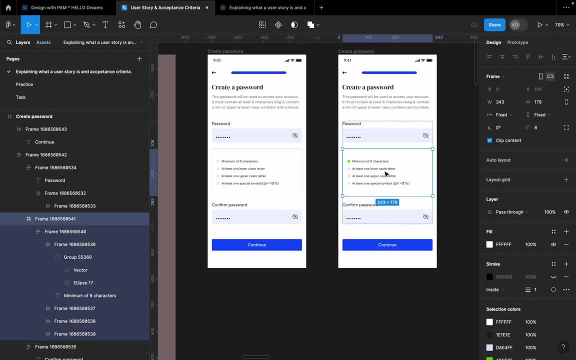 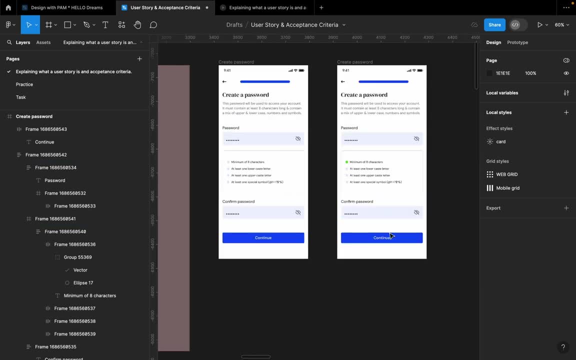 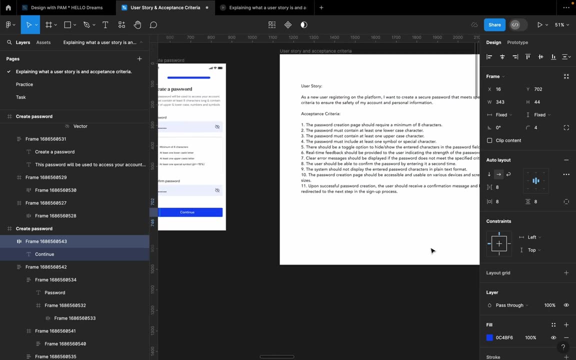 the checker is going to turn green, indicating that you have fulfilled this criteria, right? so if if you've not fulfilled this criteria, it's not going to show you that it has turned green. so whichever one do we have, the user should be able to confirm the password by entering it the second time. we already 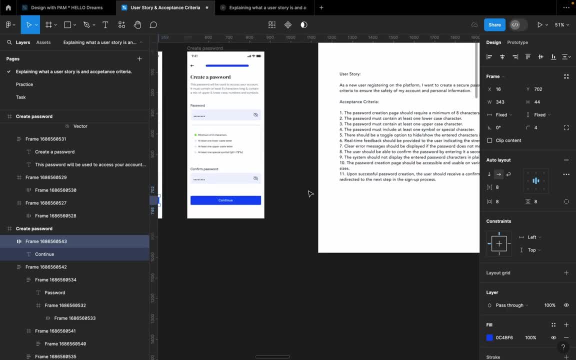 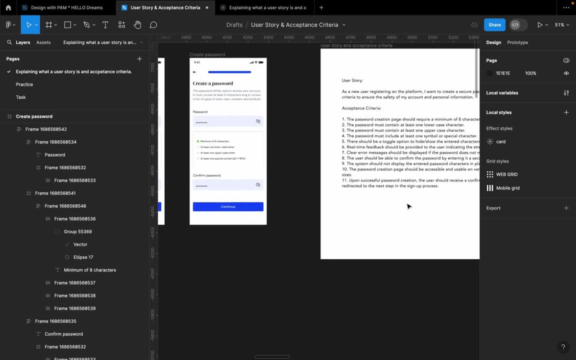 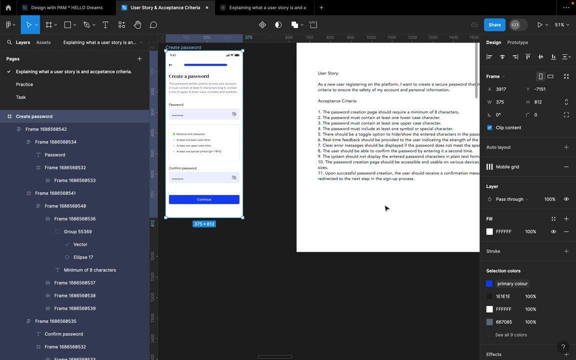 have that here. the system should not display the enter characters in plain text. we already made this available here. then the password creation page should be accessible and usable on various screen sizes. okay, this is good. um, you can walk around that if maybe there are other screen sizes you want to make provision for, and then, upon successful creation, the user should. 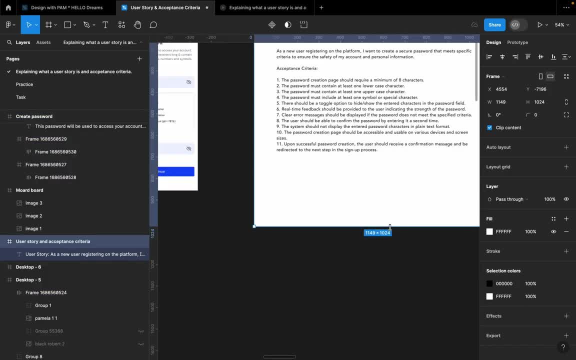 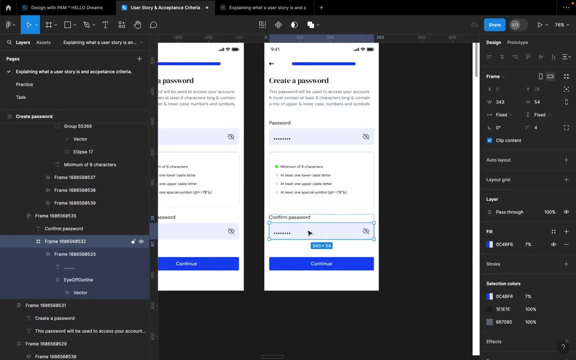 be receiving an education message and he should be redirected to the next signup page. but we're not going to treat another signup page- let's say, for instance, the first password you entered here is not the same with this one, so we can also make provision for that. let's give this a stroke and 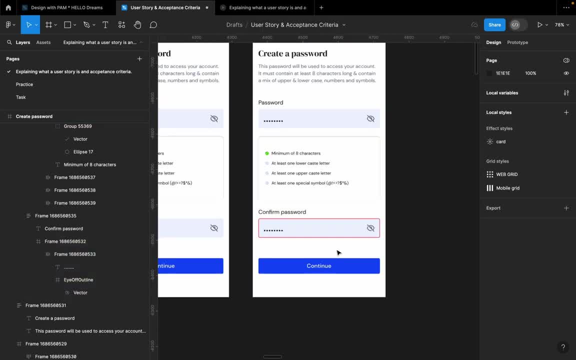 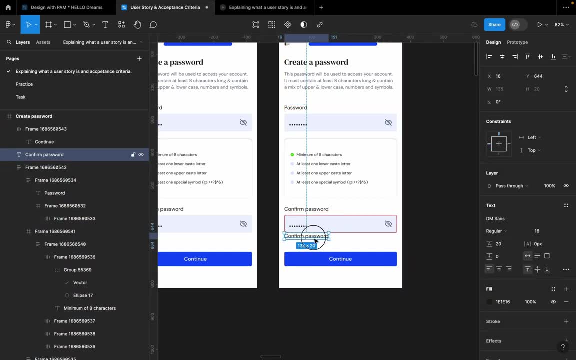 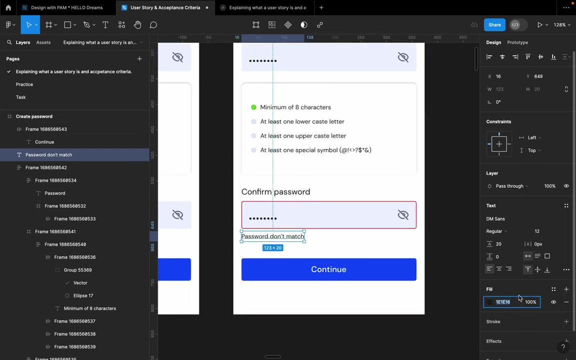 let's make this stroke a red. this place typically shows you that, oh, your password is wrong, and we can go ahead and add a test here that says: password don't match. so let's reduce this to a 12 and let's also make this a red right, so this can be an indicator that your passwords. 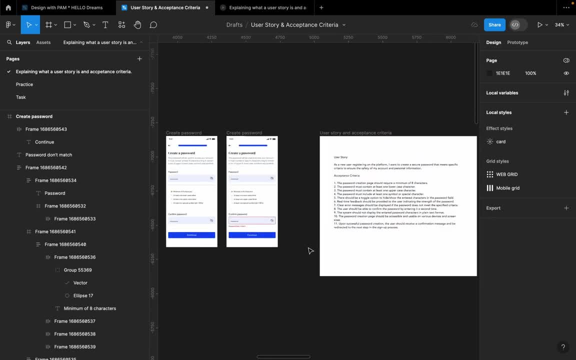 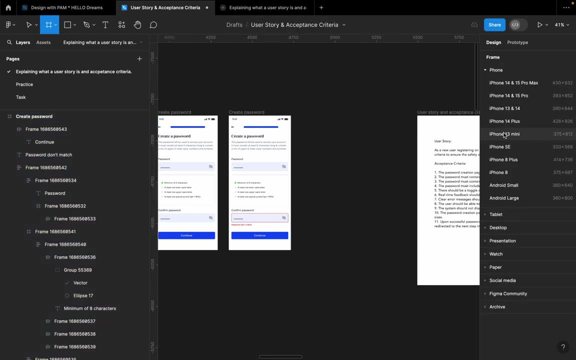 they do not match. so when you're done with this, you can also make this a red on. we can also give you a success screen to say password successfully created and proceed to dashboard. so i'm going to just click f on my keyboard, select this frame. then let's title this: 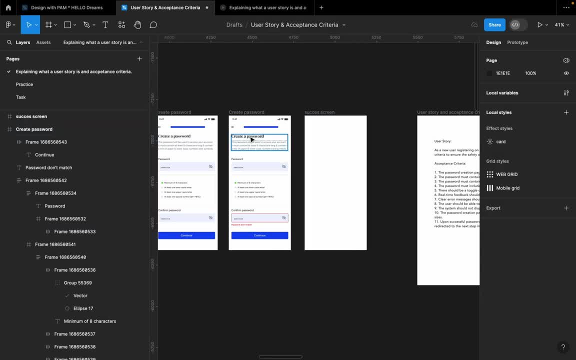 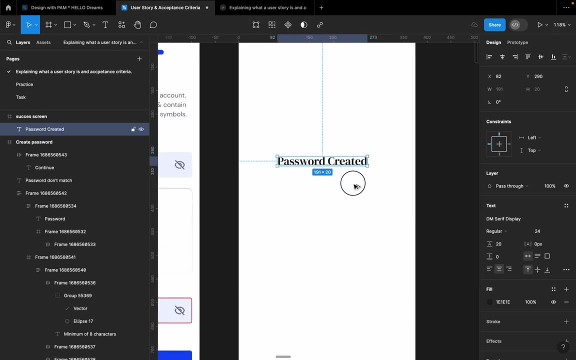 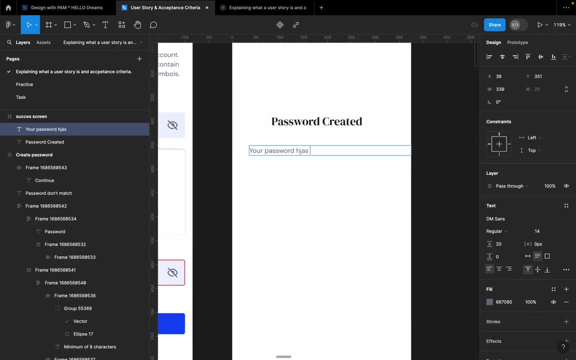 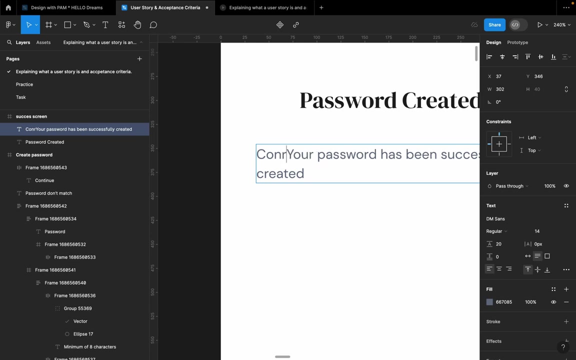 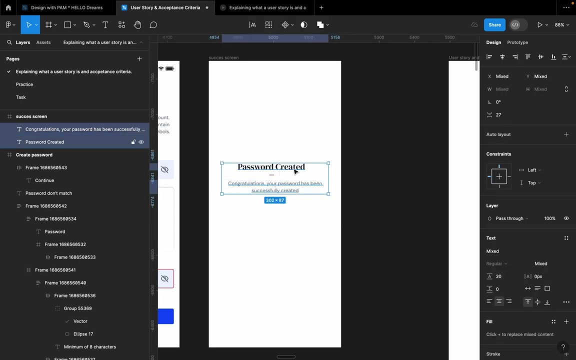 screen. so let's just pick this one here. let's say password created. so let's also take this and say: your password has been successfully created. maybe you can even say congratulations. so let's make this center line. select this to create another layout. spacing should be 28, it's. 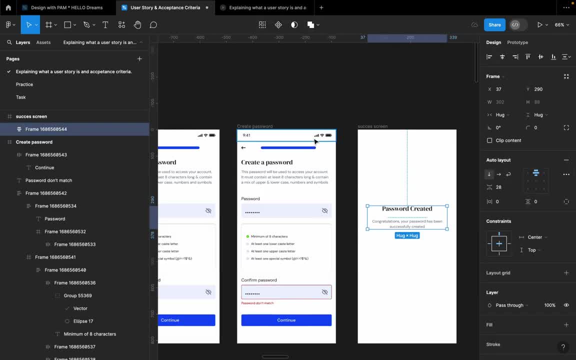 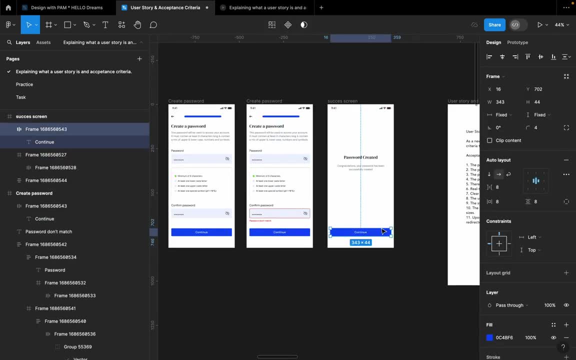 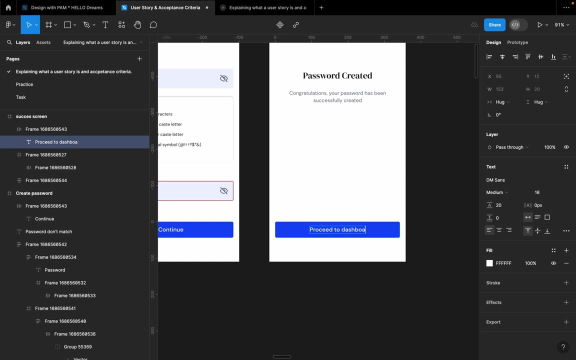 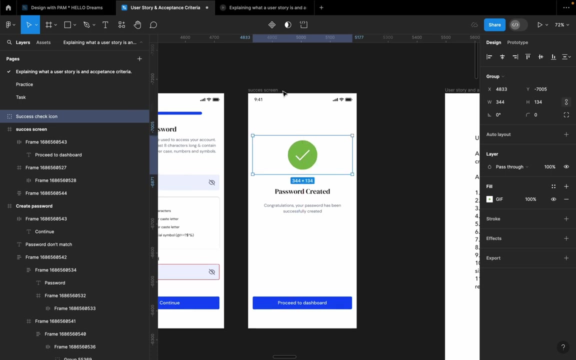 fine, it's fine going to center this. let's bring in these items that we have here. let's type this. let's say: proceed to dashboard and go further and then put some animation here. maybe this give here to say success. so what this does is: let me play it, let me preview it here. so 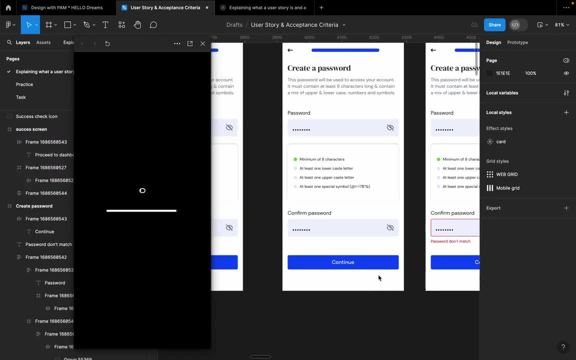 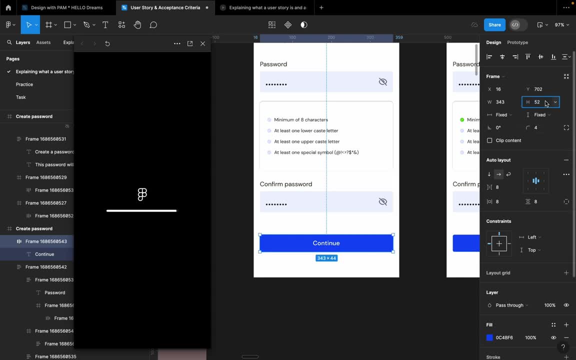 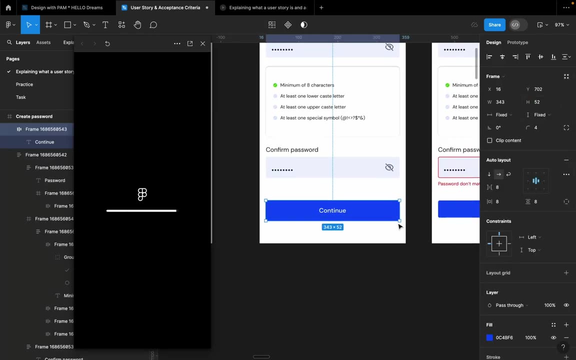 you can see it, so i'm previewing it. but while this is loading, i want us to um work on the height of this. let's change it from 44, let's say 52. i think i prefer 52. it's both. that so most times, why it takes time to previews, maybe maybe your network is not strong. yeah, 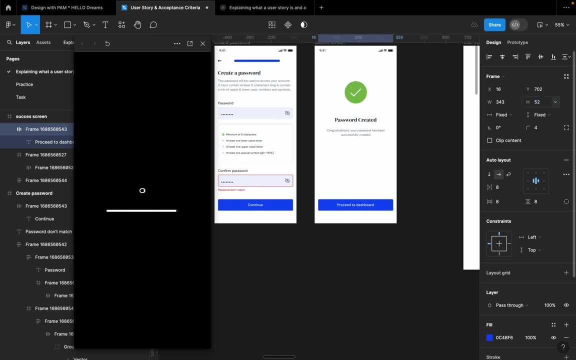 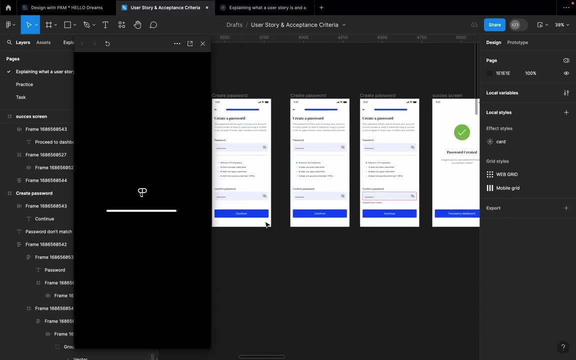 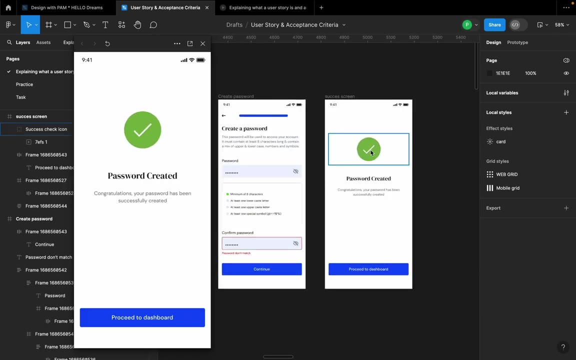 my network is not strong, making this a 52, which is fine, okay, so for this success screen, it's always good to put some kind of animation here to show that, yes, this is good, you've done, you've created your password and you can proceed to. you can proceed to dashboard. let's make this a bold. i think a bold is better, all right, so. 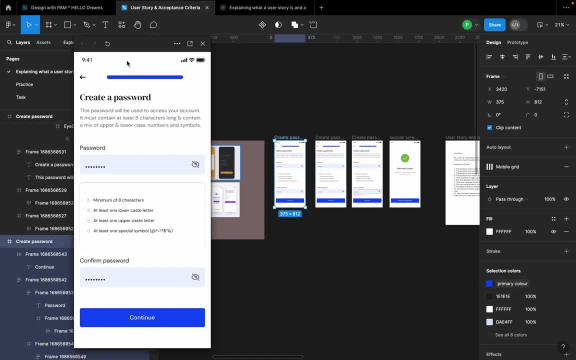 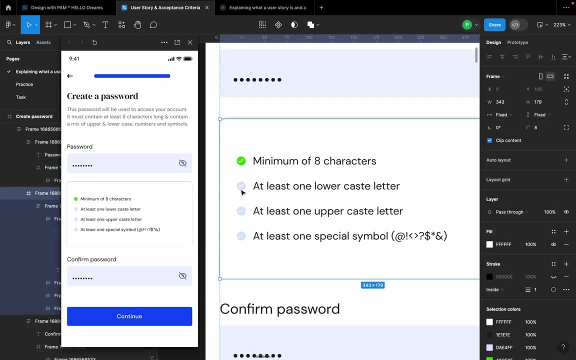 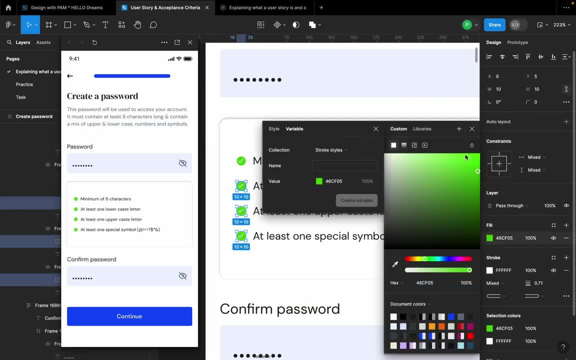 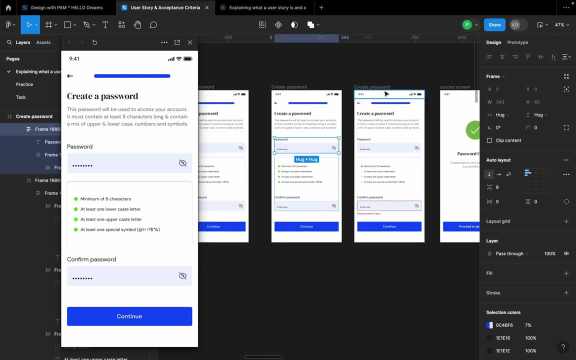 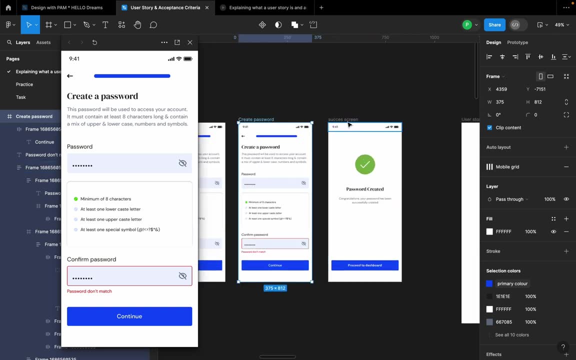 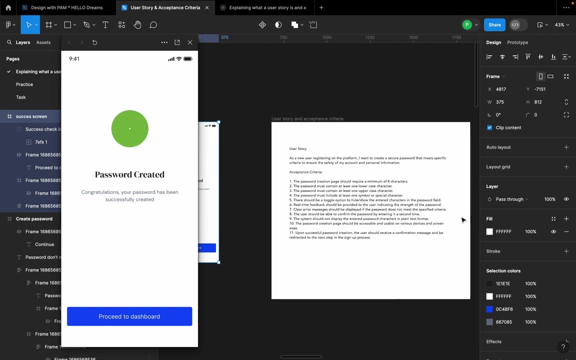 is that so? if you do that, where is my successes? i've made it look pretty easy. we'll see, but these one- she has a little, please. perfect for our annotation. see this error message and if the user has successfully created it, you get to also see this. let me know what you think and if you have any questions, leave it on the comment section. 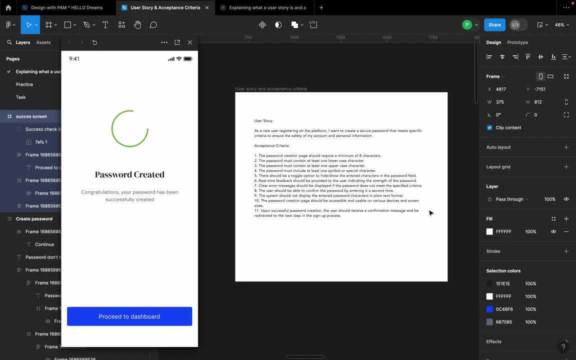 if you found this video helpful, please subscribe to my youtube channel. thank you.